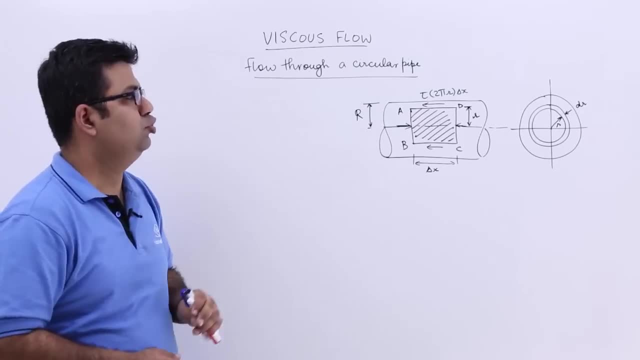 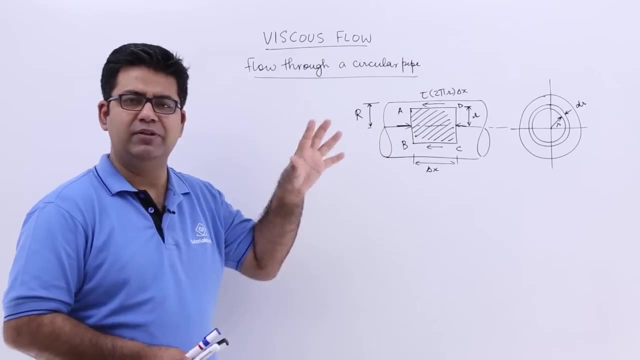 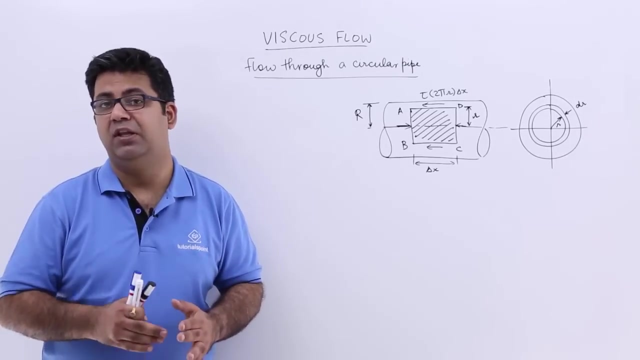 Now let's talk about the concept of viscous flow through pipes. So this is the first topic on this chapter, which is the flow through a circular pipe. Now, what is viscous flow? Viscous flow happens when the viscosity of the fluid is very high, or the velocity of 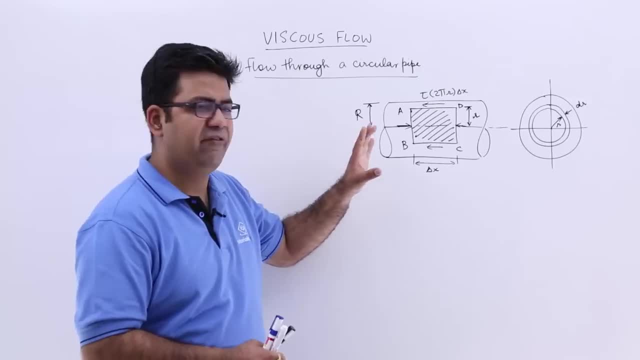 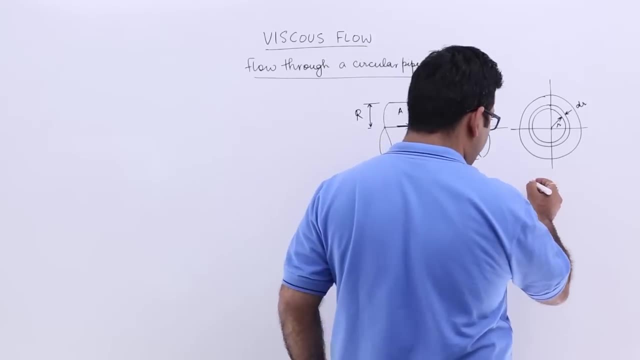 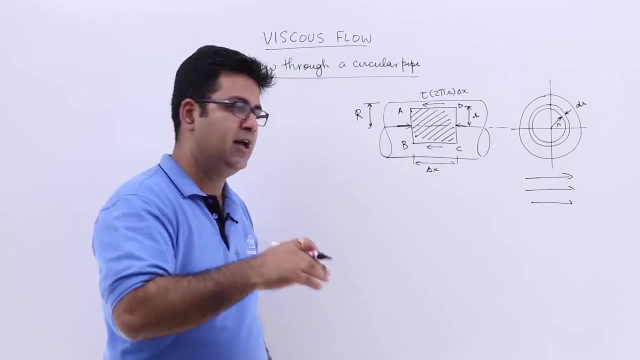 the fluid flow is very, very low. When the fluid is flowing in a very, very slow velocity, then the flow or the fluid is moving in layers like this, And due to this motion in layers there will be some velocity gradient and due to this there will be some production of shear. 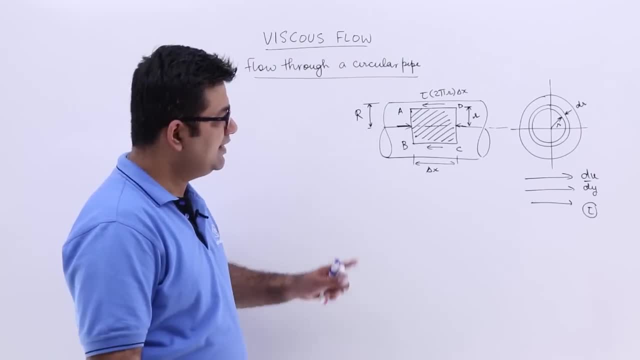 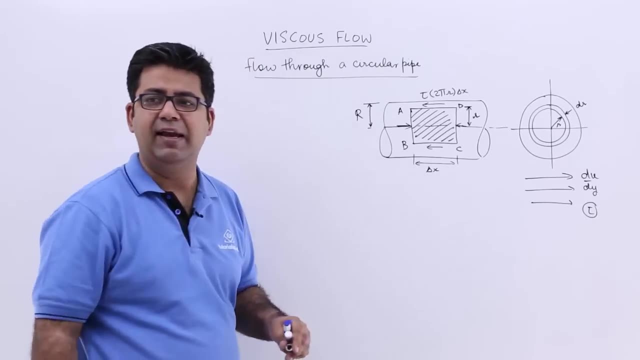 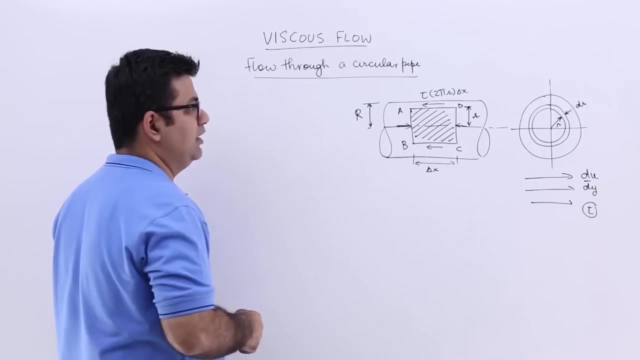 stress. So in this we have to find out that what is the pressure drop in this pipe when a very highly viscous fluid flows through the pipe? Okay, so this is a very simplistic diagram shown to you. So this is a pipe through which 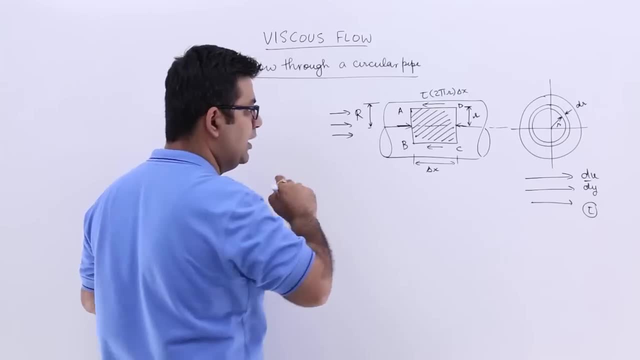 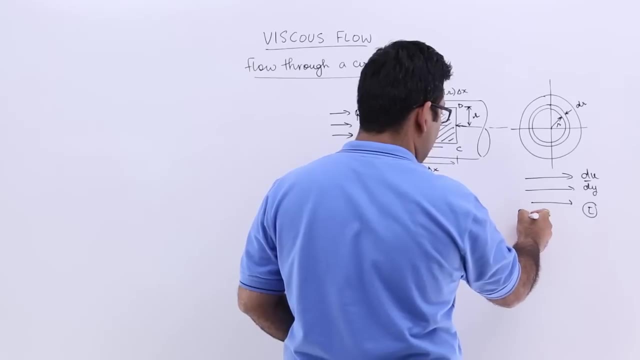 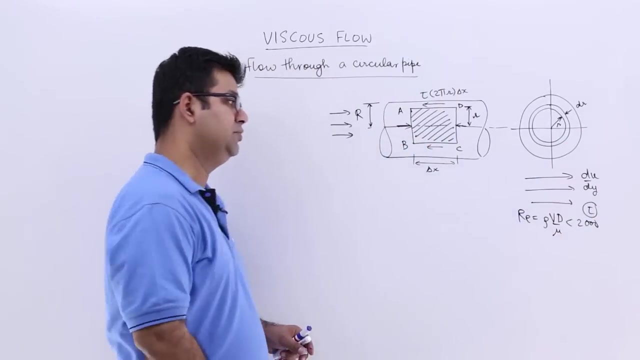 a very highly viscous fluid is flowing Now. the viscosity, or I would say this kind of flow will only occur if the Reynolds number, which is rho into V, into D upon mu, is less than 2000.. Okay, so it's a very highly viscous flow. 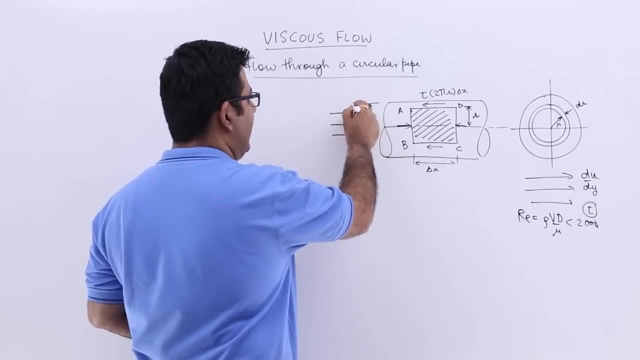 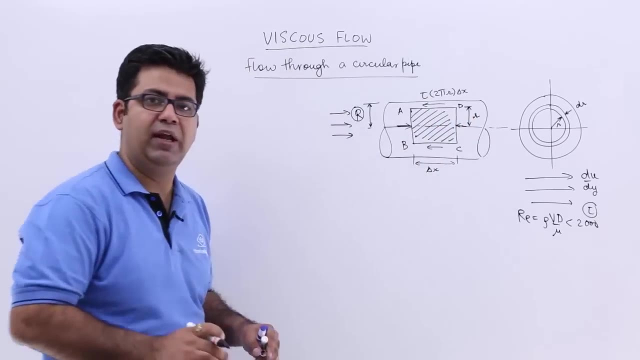 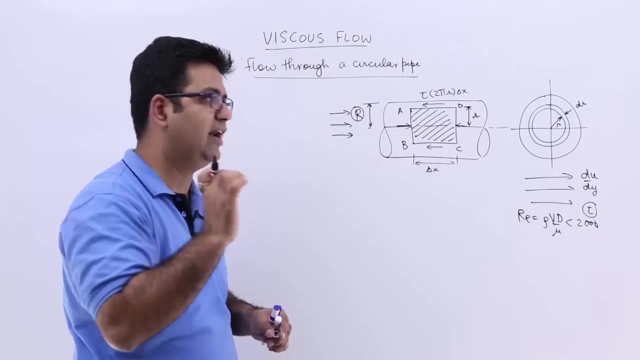 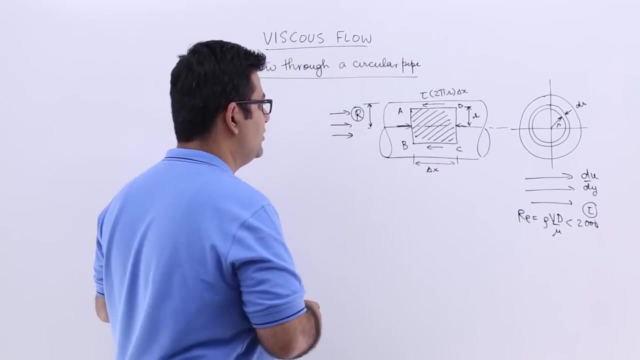 And let's assume that the pipe has a maximum radius of capital R. Alright, so we assume a small fluid element. Now this fluid element, ABCD, which is of radius small r, is sliding inside a cylindrical element which is of the radius r plus dr. Okay, so what happens is: 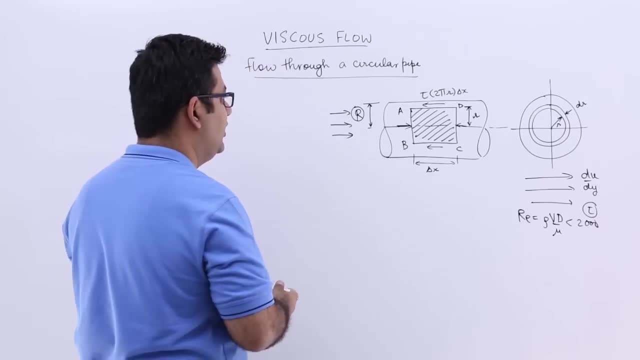 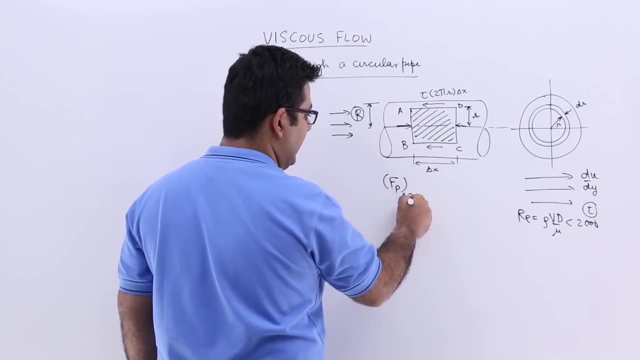 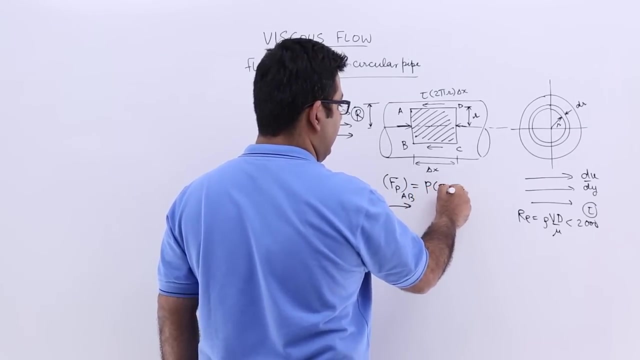 on this: on the face AB, the pressure force which is the force of the pipe, which is the force which is acting. So the pressure force which is acting on the side AB, and this would be in the right direction. This would be pressure into the area which is pi? r square. On the other hand, the pressure 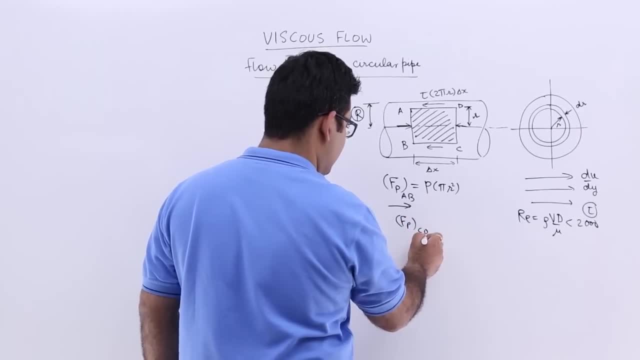 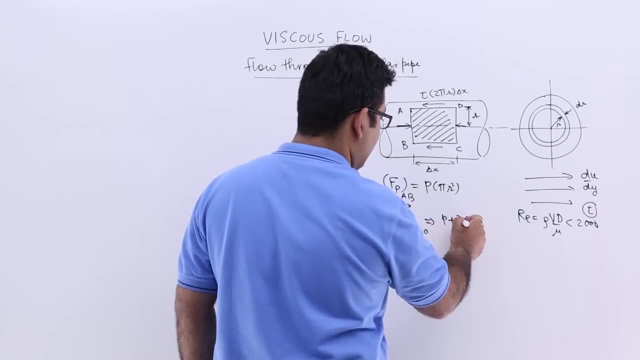 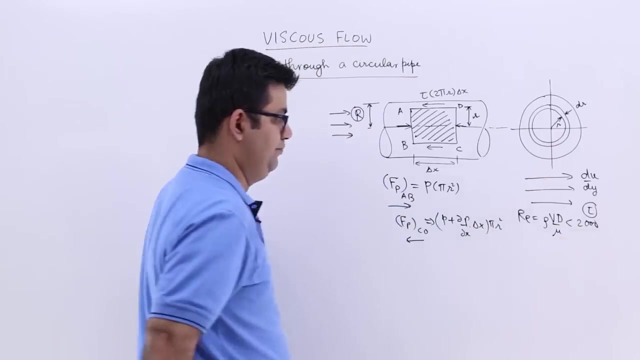 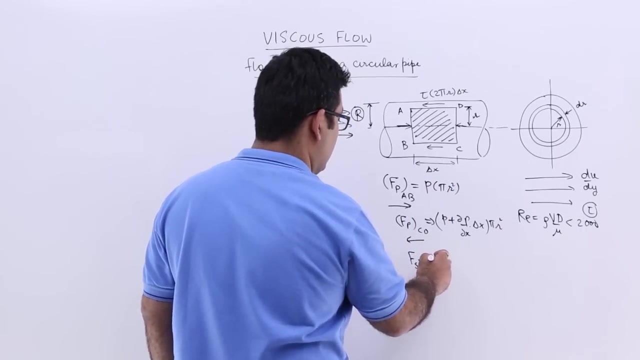 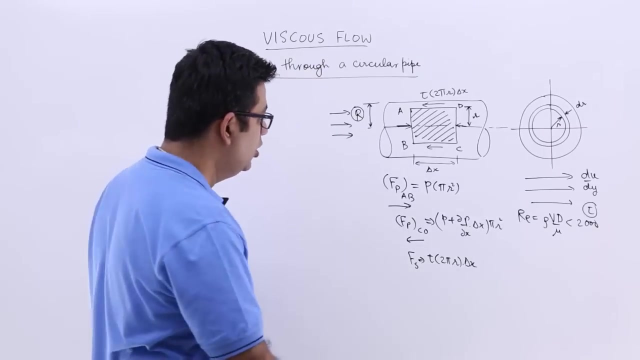 force on the face CD. this would be in the left direction and this would be P plus curly P. by curly x, x into delta, x into pi r square, okay. and there is some production of shearing force, so shearing force is tau into 2 pi r into delta x, okay. so because there is no acceleration given, 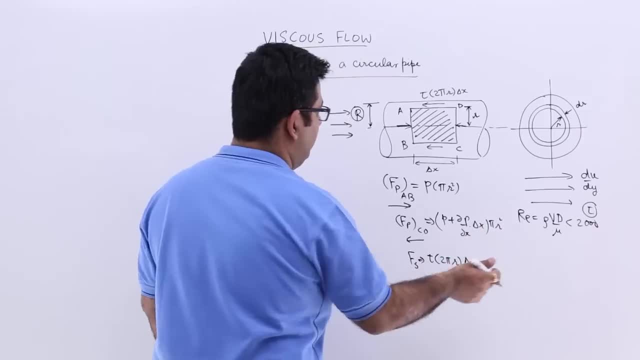 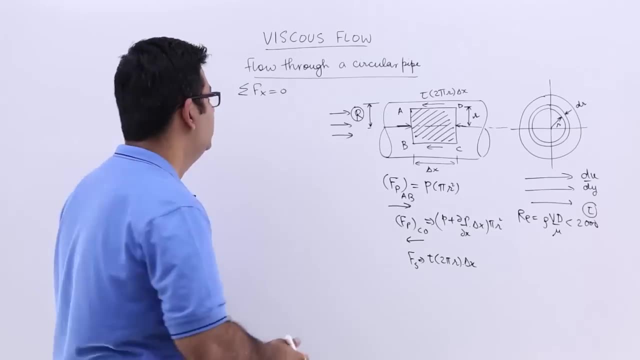 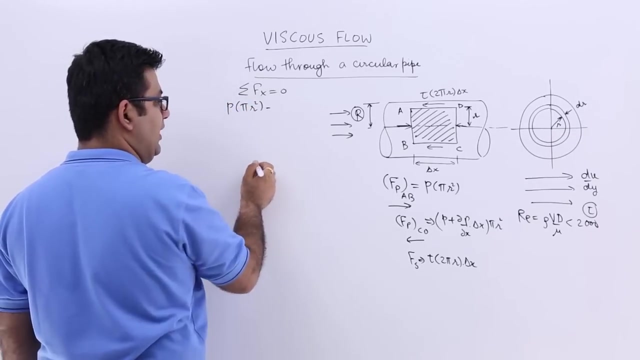 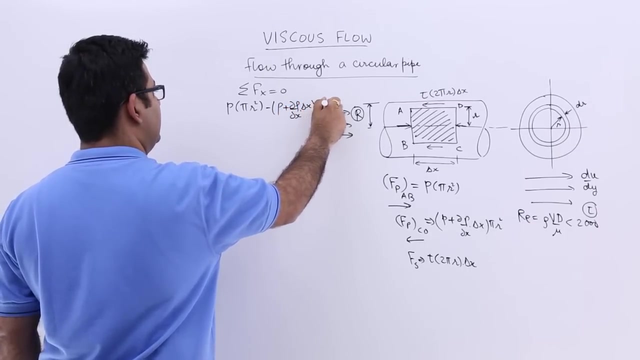 to the fluid. so the net force would be 0. so you will write down summation f x 0 and there is no force in the y direction. we will just take the x direction. so you will have p into pi r square minus p plus curly p by curly x into delta, x into pi r square minus 2 pi. 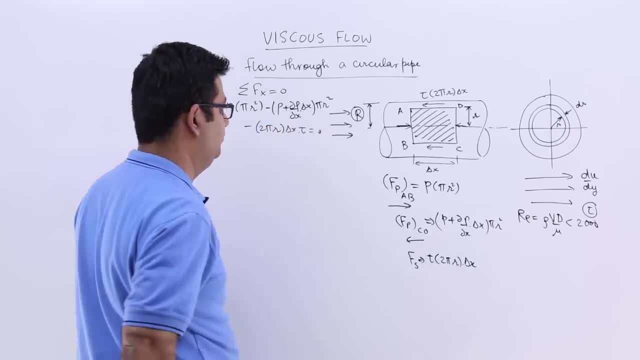 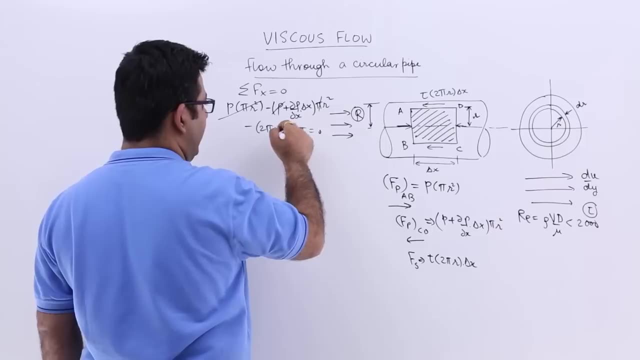 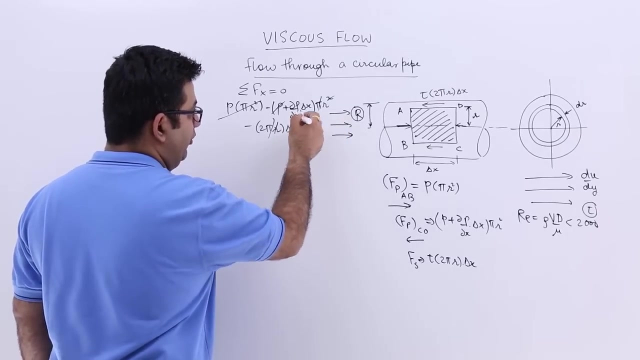 r into delta x square. Okay, x into tau is equal to 0. from here, I can straight away strike of this part, and then I can strike of pi, and then I can strike of r and this r. so we are left. before I do that, I can also. 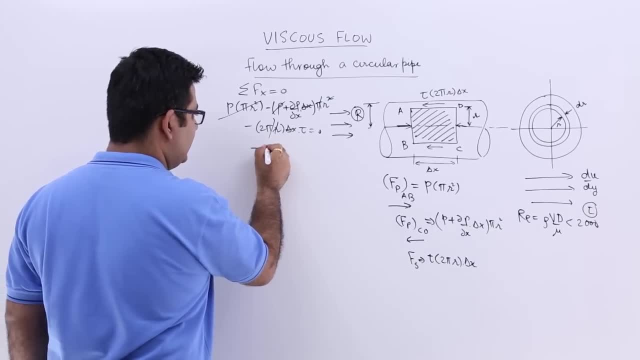 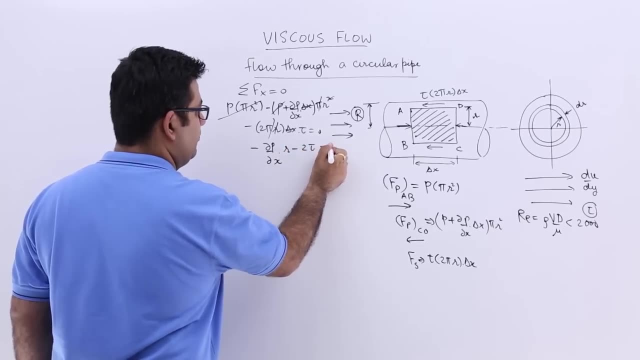 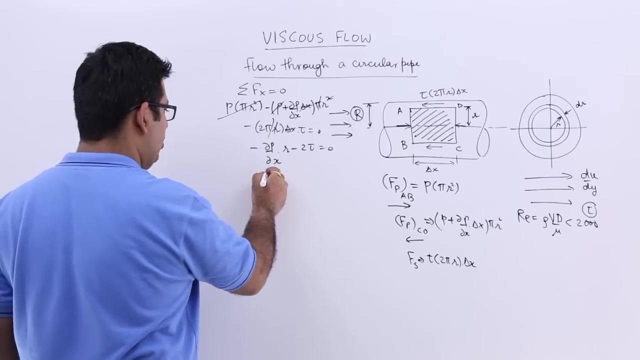 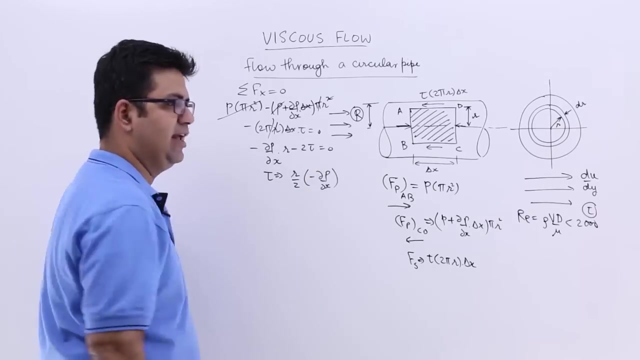 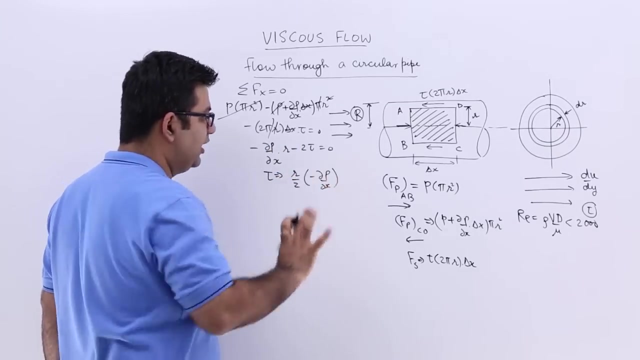 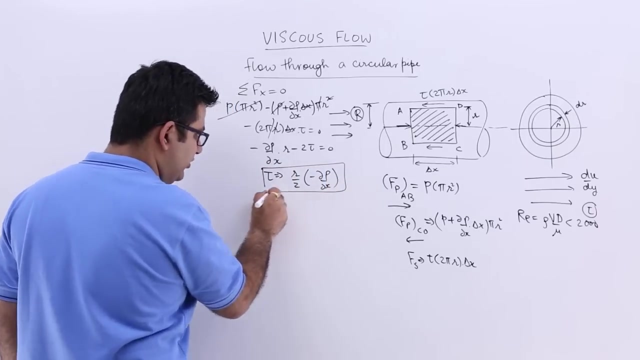 strike of delta x. so now I have minus of curly p by curly x into r minus 2 tau equal to 0. okay, so from here I can find out the value for tau. so tau will be equal to r upon 2 into minus curly p upon curly x. so this tells us the shear stress distribution in such a flow. now the pressure gradient is constant throughout the pipe. okay, this means that the value of shear stress in this kind of a flow will vary linearly with respect to the pressure gradient. 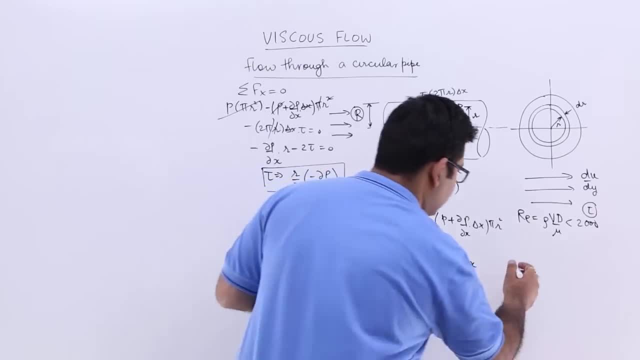 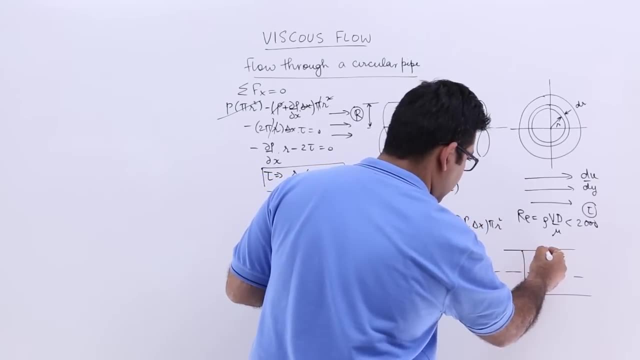 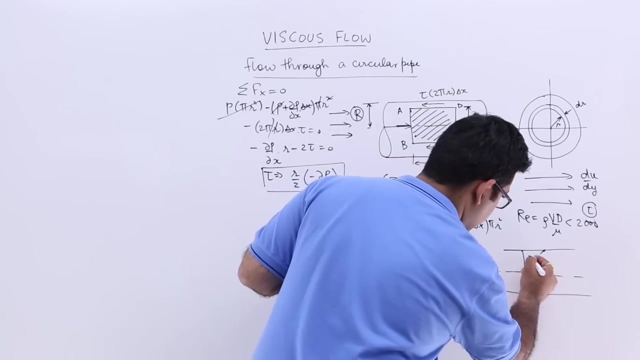 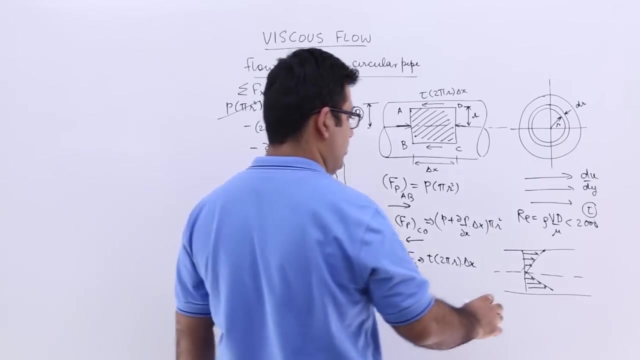 intersect to the radius. okay, so if I draw the shear stress distribution, this is, let us say, the pipe. alright, your distribution of shear stress would be somewhat like this. so this is how the shear stress is distributed. I can say: this is my shear stress, okay. 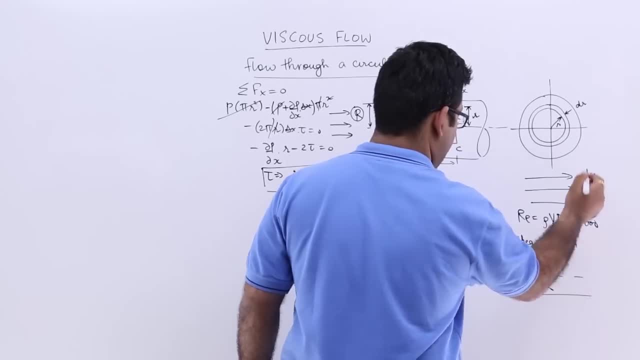 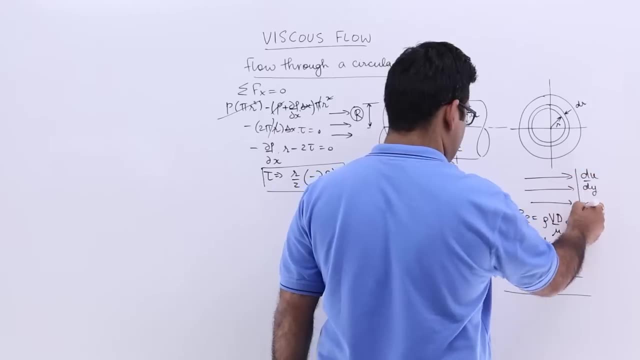 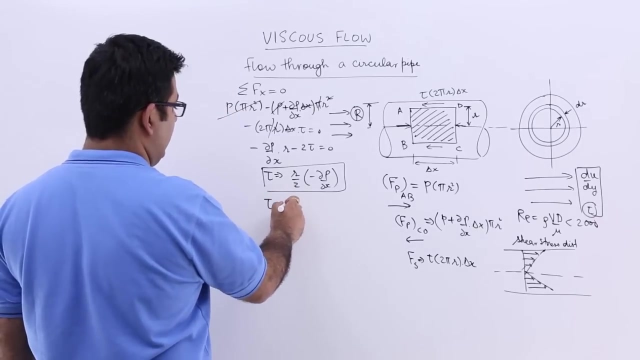 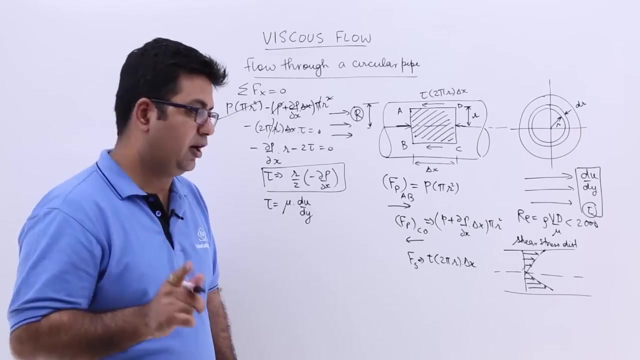 Okay, Thank you. Okay, fine distribution. okay, so my tau is taken care of now because there is a production of shear stress, so I can apply the law of viscosity, so I can say tau is equal to du upon dui. is that right now? there is a very important thing to understand over here when we calculate. 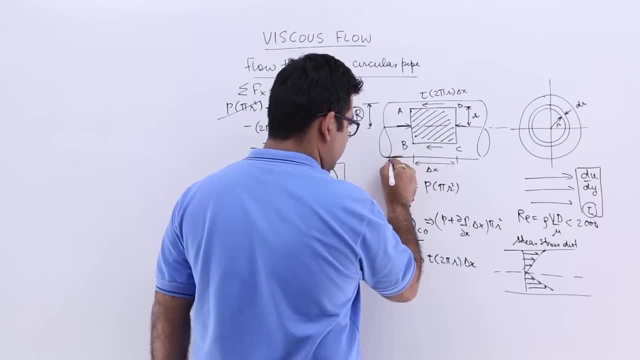 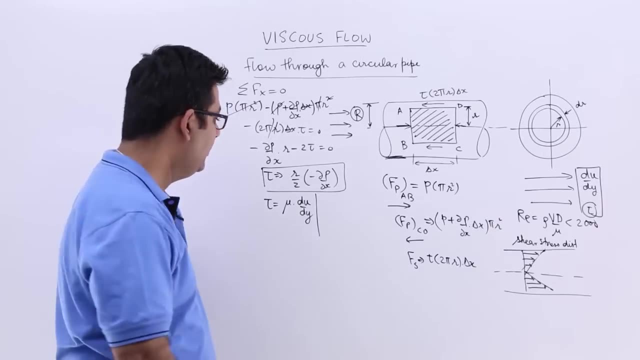 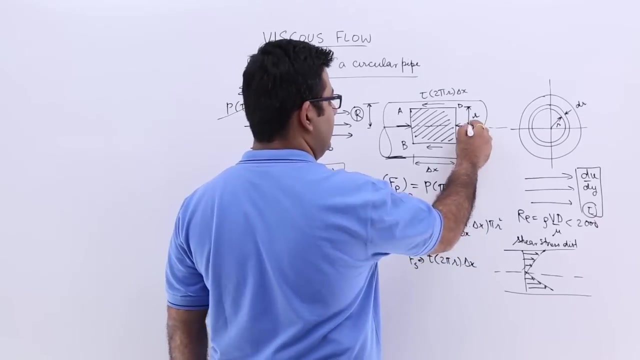 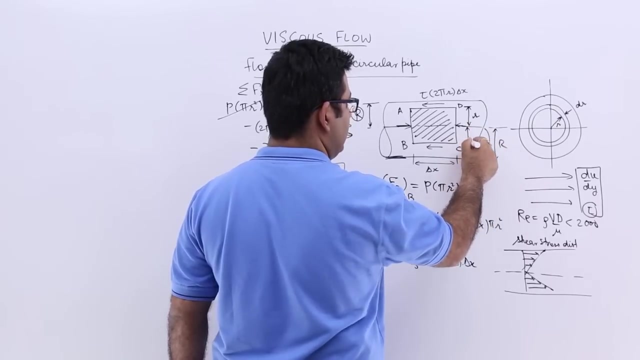 this. this is calculated from the bottom surface of the pipe, okay, but we are talking about this fluid element, okay. so for this I would have to take dr instead of dy. so if you look at this, this is r and this much is r, so y would start. 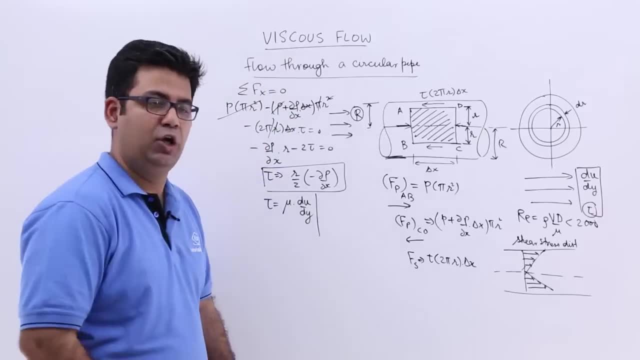 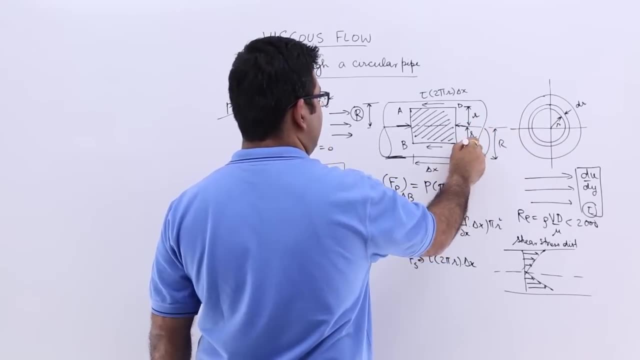 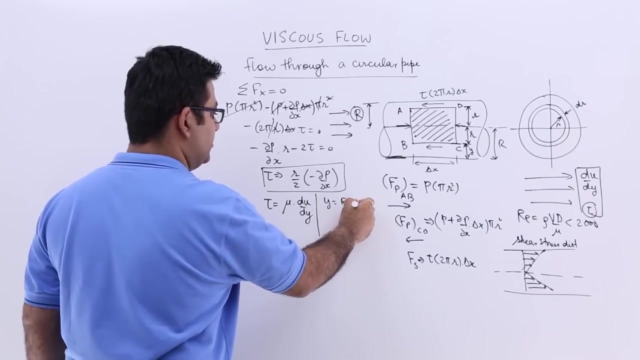 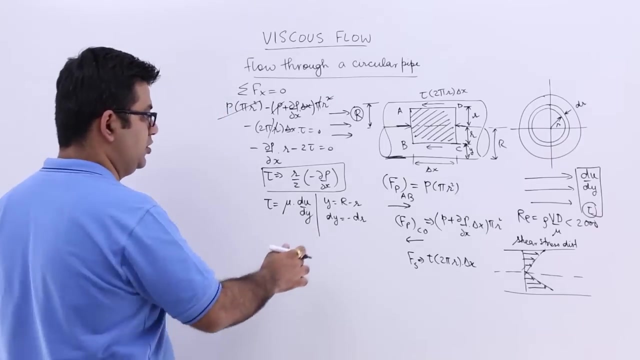 At this particular point, not at the bottom of the pipe. so the value of y is capital R minus small r. this is your y. okay, so I would say that y is capital R minus small r. so I can say dy is equal to minus d small r, because capital R is a constant value. so this is constant. 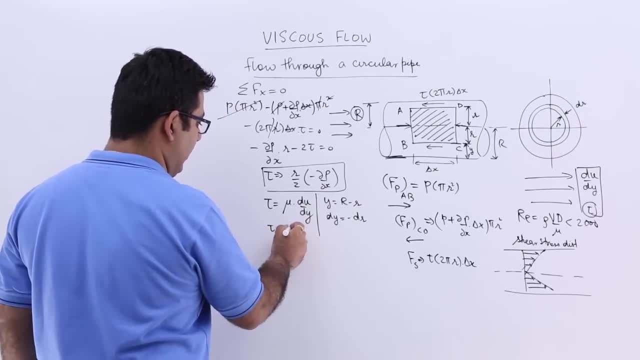 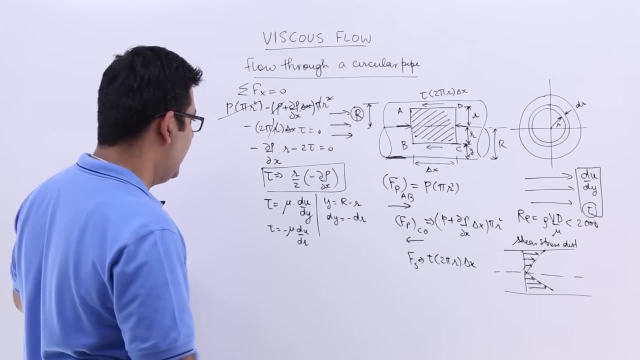 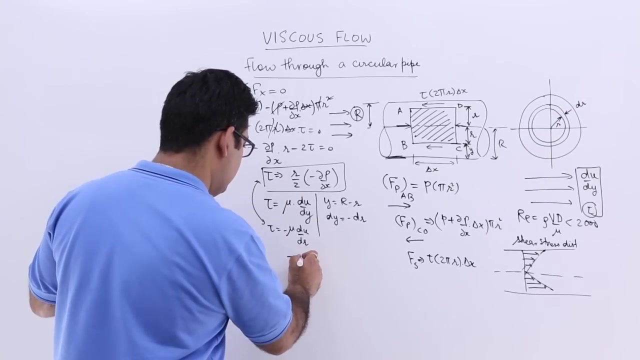 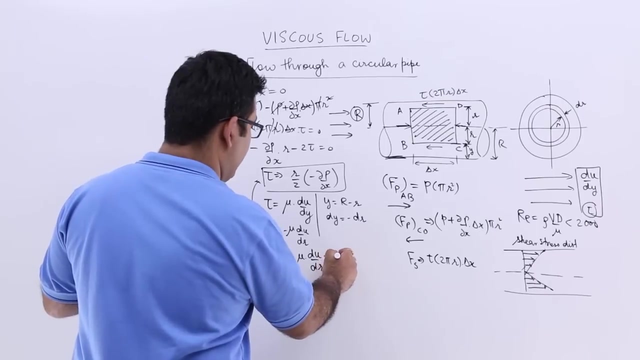 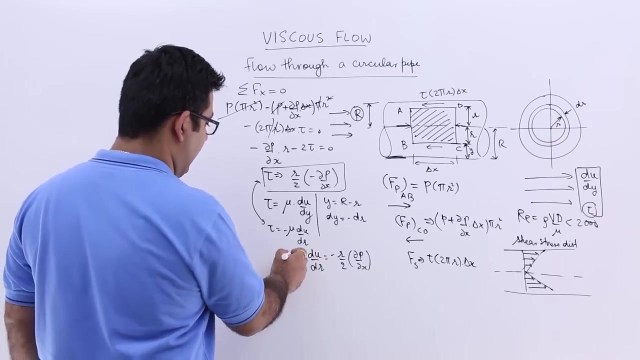 you get this so I can put down: tau is equal to minus mu dui, So from here I can equate these two equations. so when you equate you get minus mu du upon dr- this is equal to minus r by 2- into curly p upon curly x. I can get rid of this and I'll 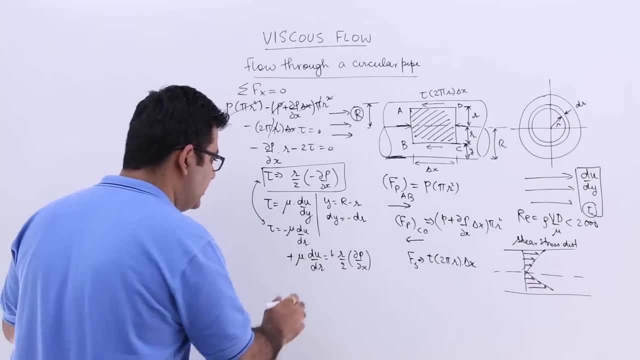 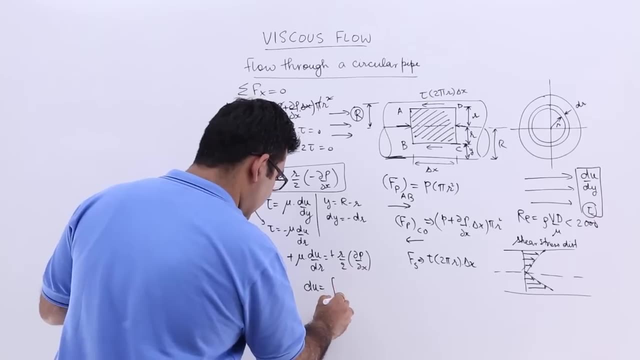 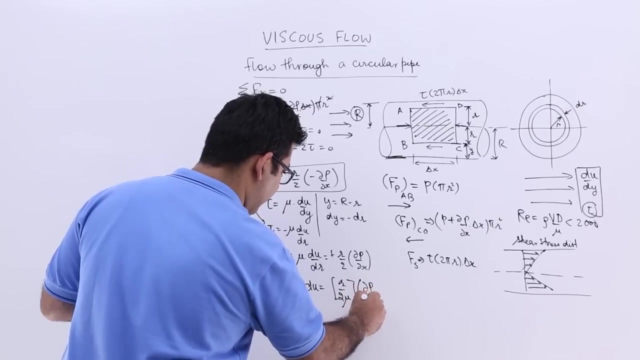 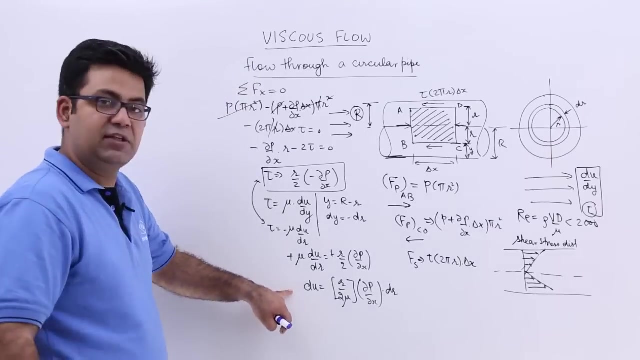 have positive on both sides. now, from here I can say that du, du is equal to. I can say this is equal to R upon 2 mu into curly p upon curly x into dr. so this is the change in velocity. okay To find out. 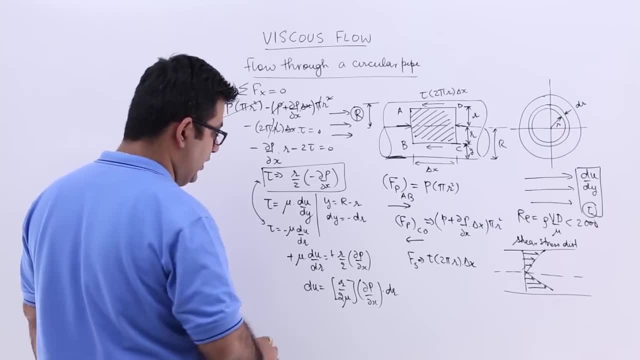 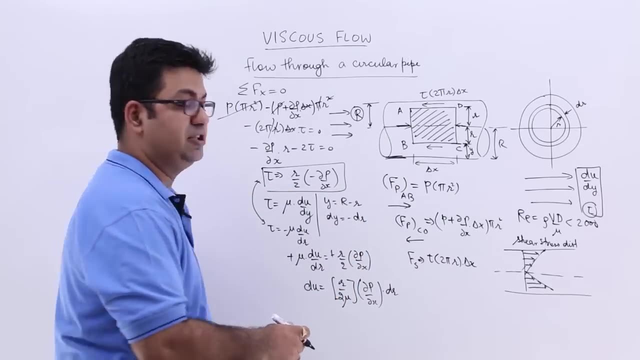 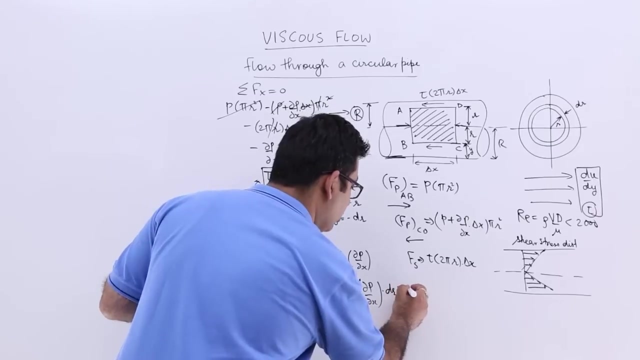 To find out out the maximum velocity I would have to, or I would say the velocity for this, or to find out the velocity distribution, I will have to integrate this. So to integrate after integrating, you would get a value which is u. now we are integrating. 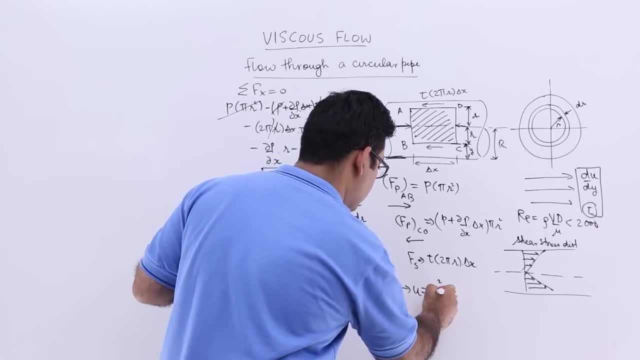 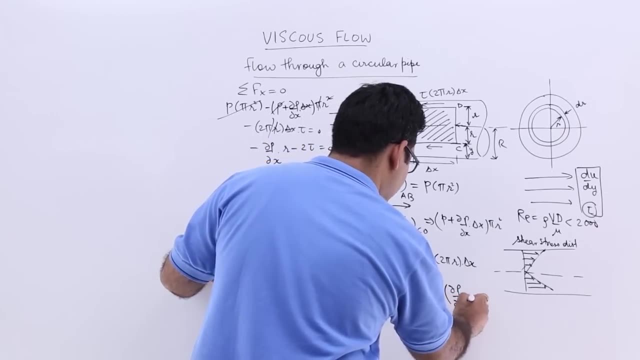 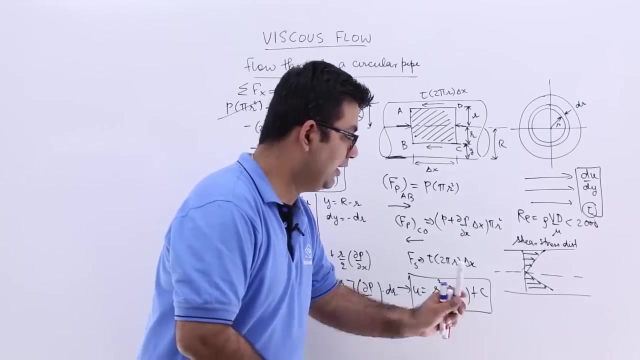 with respect to r. so you will get r square upon 4 mu into curly p upon curly x plus c, where c is the constant of integration. Now we want to find out that c so as to get a picture of how the velocity is varying. okay, 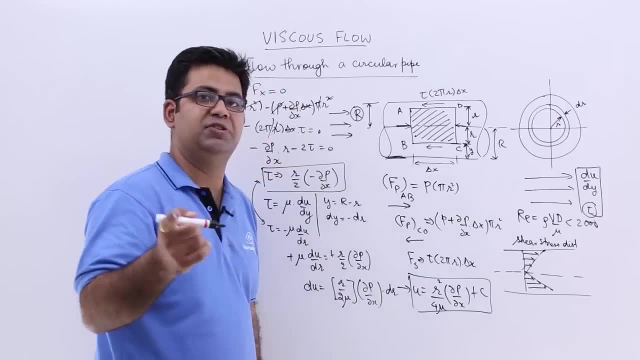 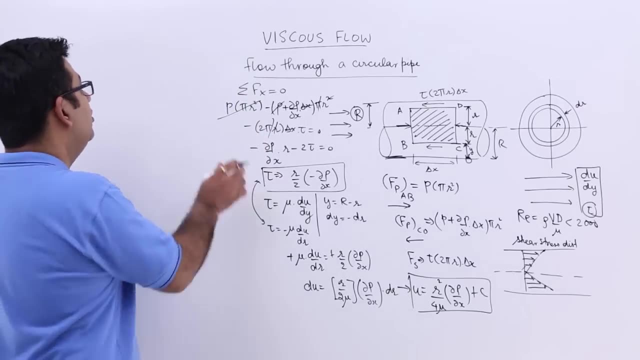 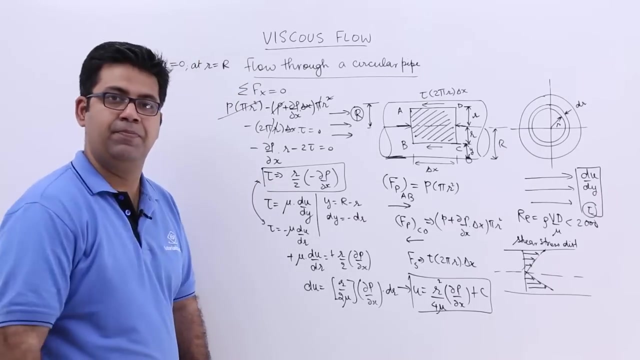 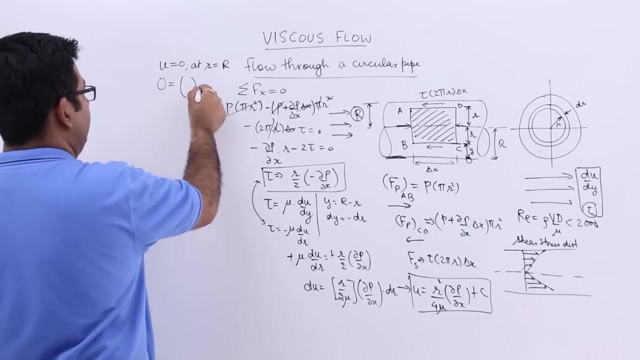 Now, if you look at this, the value of velocity becomes 0. Now when the radius becomes capital R, so u is 0 at small r, equal to capital R, right. So when you put the value over there it becomes 0 into this plus c. so the value of capital. 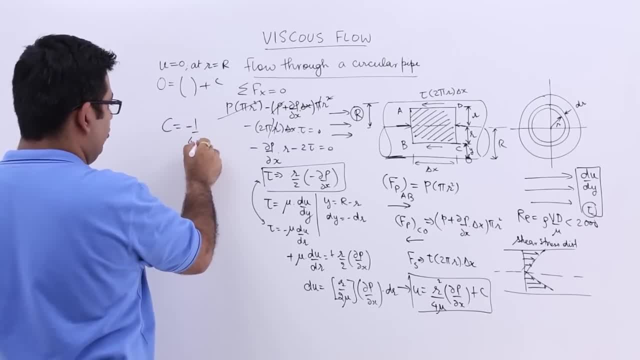 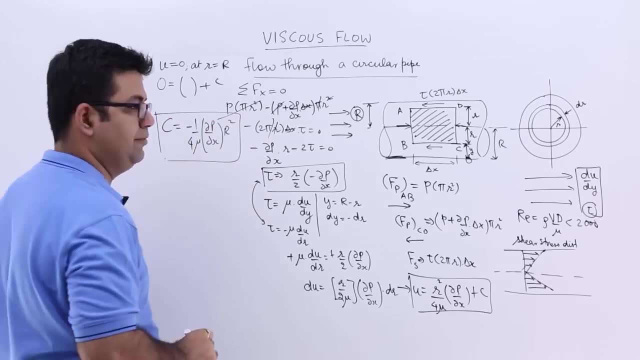 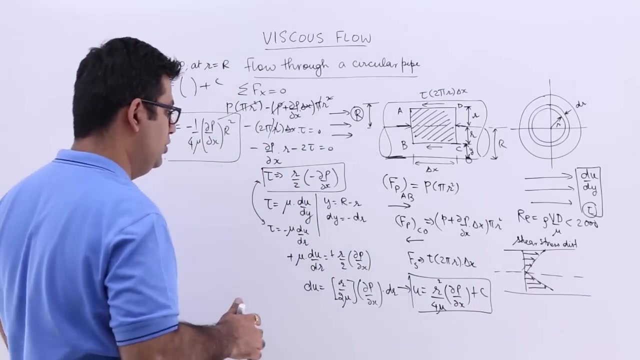 c becomes minus 1 upon 4 mu into curly p, by curly x into capital R square. So this is c. Now put this value of c over there and you will get the velocity distribution for this kind of a flow. and that will be. I will write it down over here. 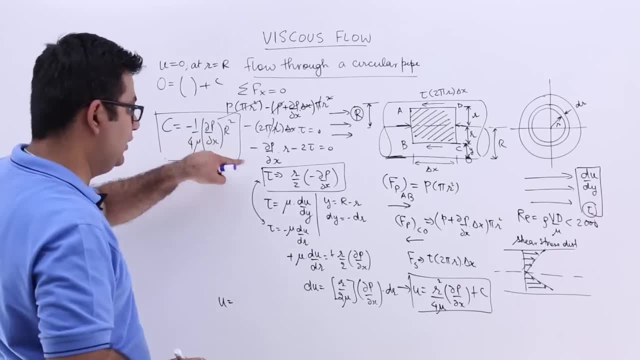 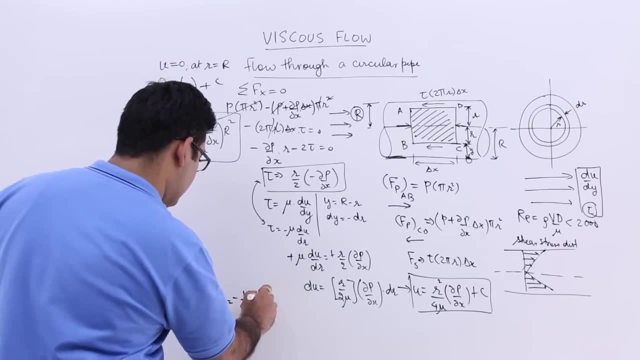 So u is equal to when you put capital R square. I can put minus 1 by 4 mu, curly p upon curly x into capital R square. So this is c. Now put this value of c over there and you will get the velocity distribution for this. 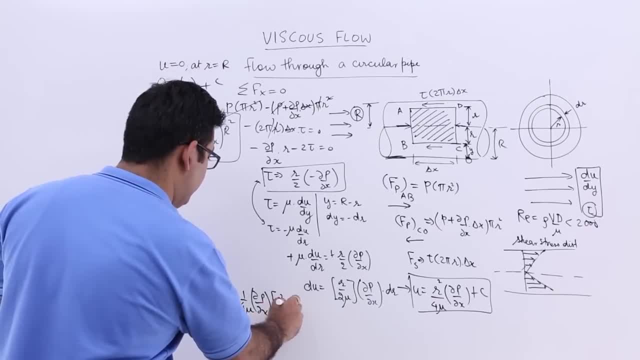 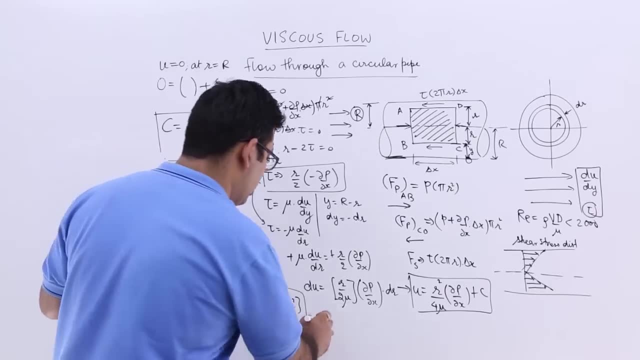 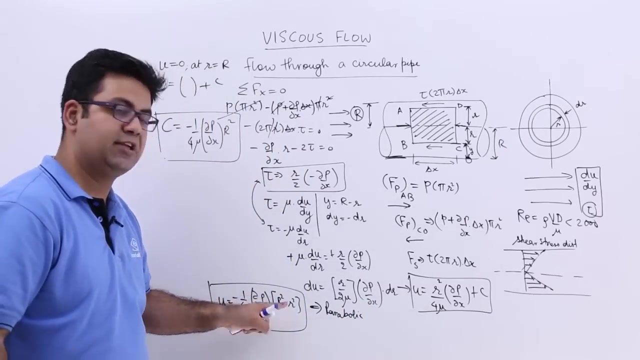 kind of a flow, and that will be. I will write it down over here. So u is equal to capital R square minus small r square. So this is how the velocity is varying. This clearly shows that the velocity distribution is parabolic, because small r is varying at. 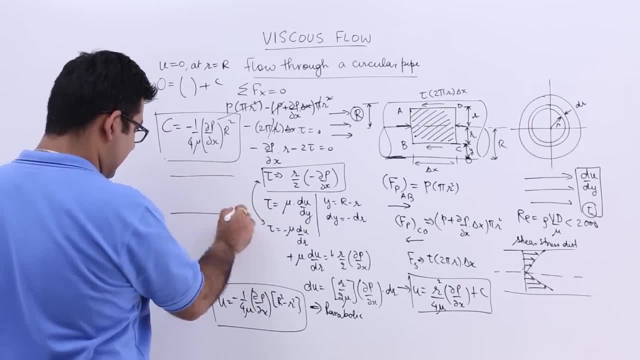 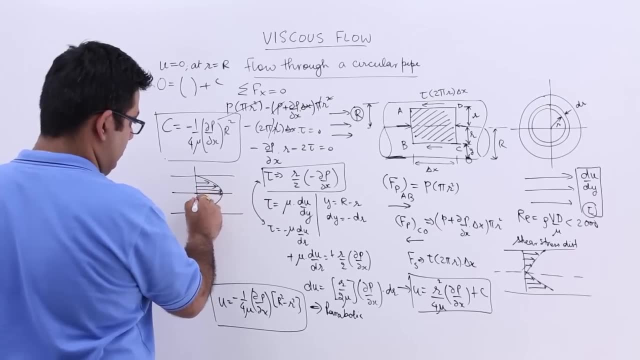 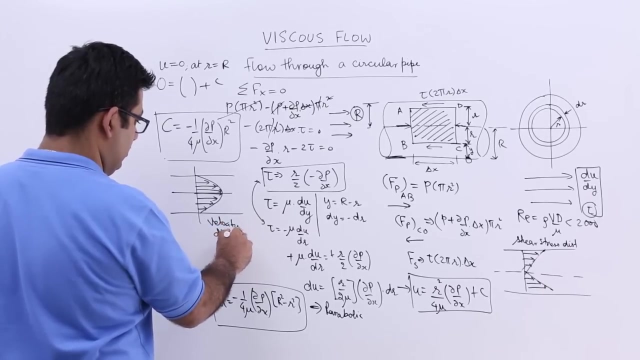 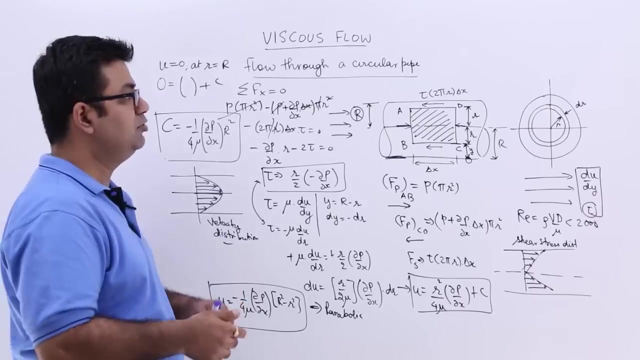 the power of 2.. So this would be like this: This is how the velocity is varying, So I would say this: So this is the velocity distribution. Okay, now the next part is to find out the maximum velocity, and then we will have to find 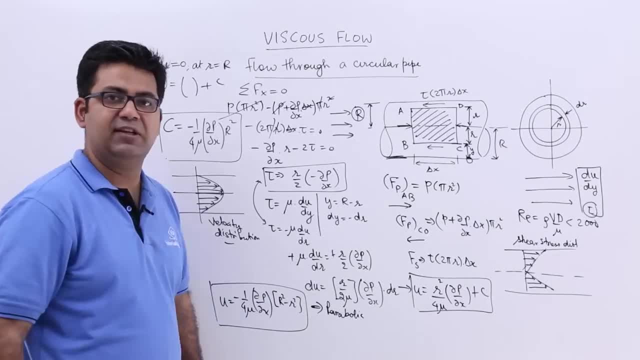 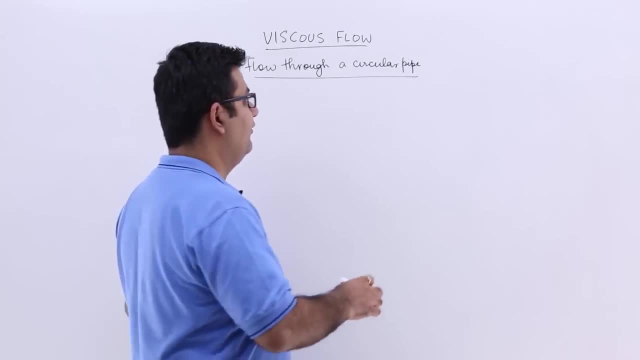 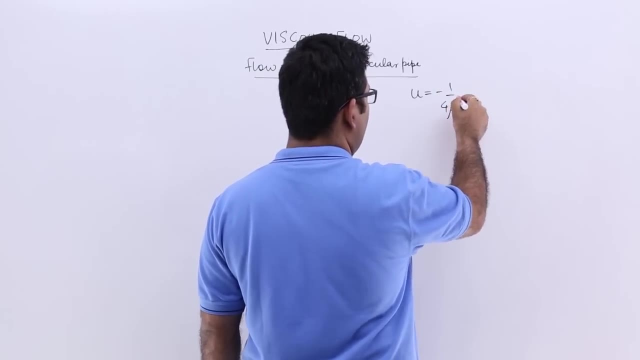 out the average velocity. So to move further in this analysis, let us make some space for writing. So let us write again the velocity distribution, So you will have u. So u is equal to minus 1 by 4 mu into curly p upon curly x, into capital R square minus. 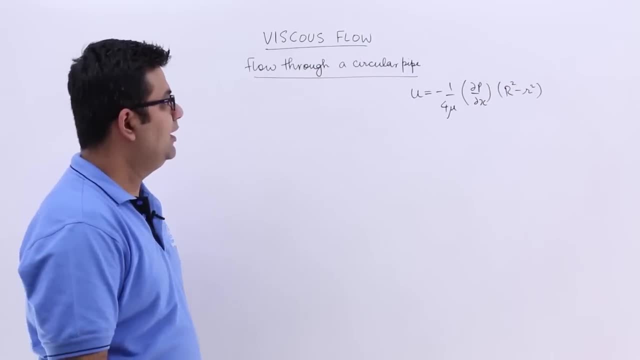 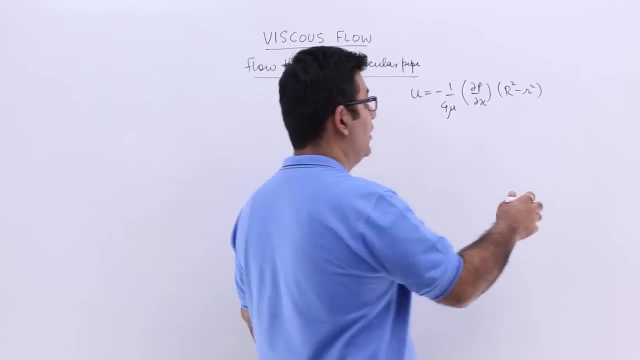 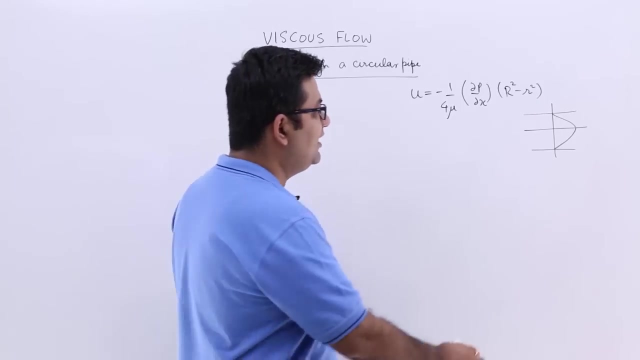 small r square. So that is the velocity distribution. Okay, let us find out the maximum velocity. So maximum velocity will occur at small r equal to 0.. That is, if you remember the you know velocity distribution. it was something like this, Okay. 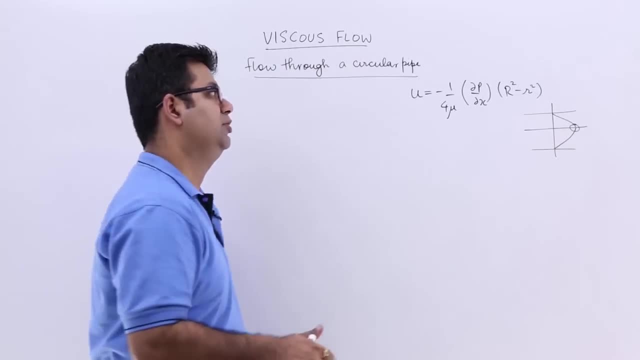 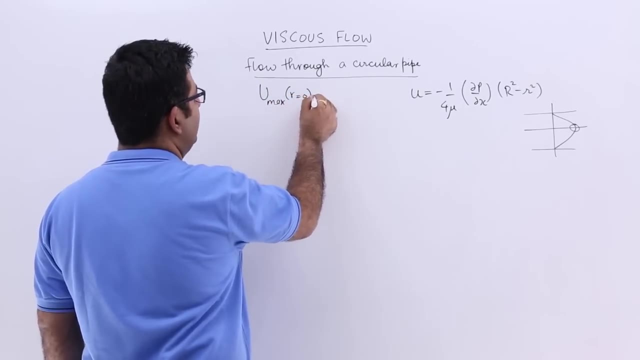 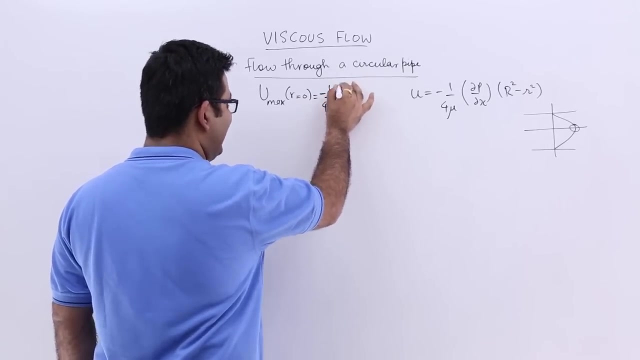 So at small r equal to 0 you are going to have your maximum velocity. So let us say that is u max, which is at small r equal to 0, and the value becomes minus 1 upon 4, mu, curly p upon curly x into capital R square. 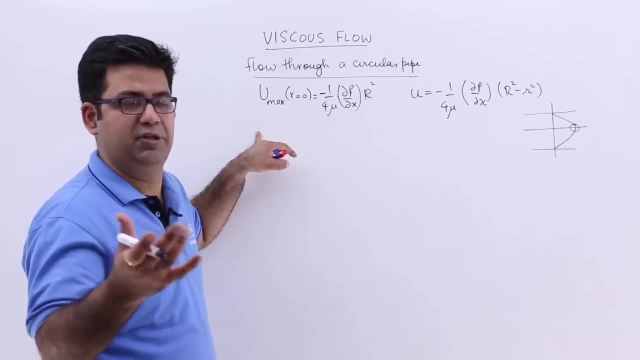 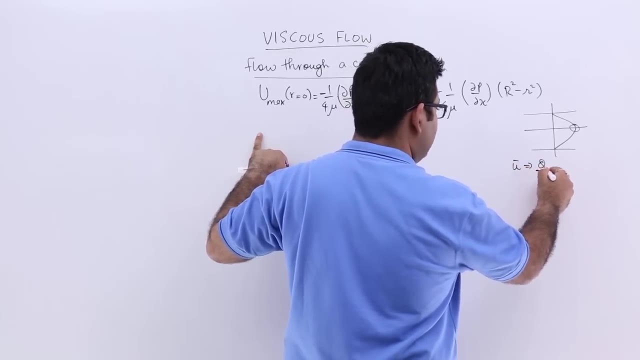 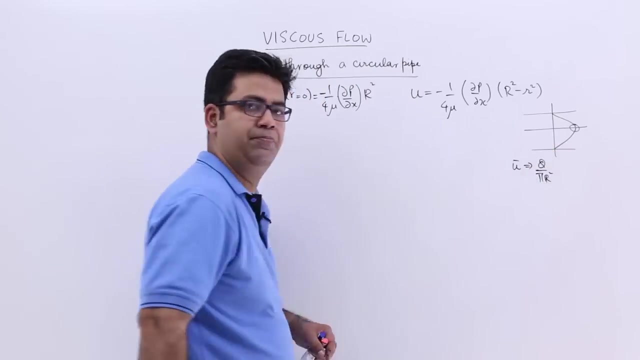 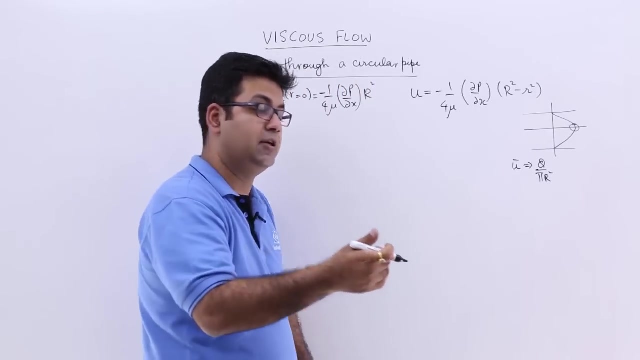 That is your maximum velocity, So let us find out the average velocity For average velocity. that is u bar. Okay, I will divide the discharge by the cross section area of the pipe, Okay. So let us find out discharge first. To find out discharge, let us take that section, that, so this discharge through that section. 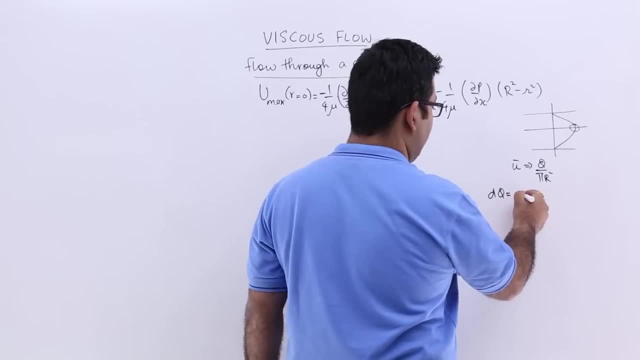 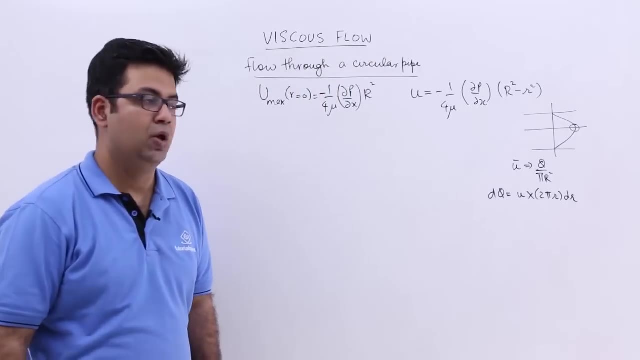 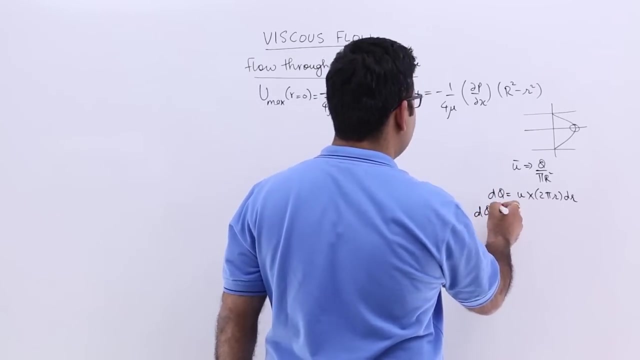 would be dq, which is equal to the velocity, u into d, volume, which is 2 pi r into dr. Okay, I will put the value of u So u from this equation. so you will get: dq is equal to minus 1 upon 4 mu into curly p. 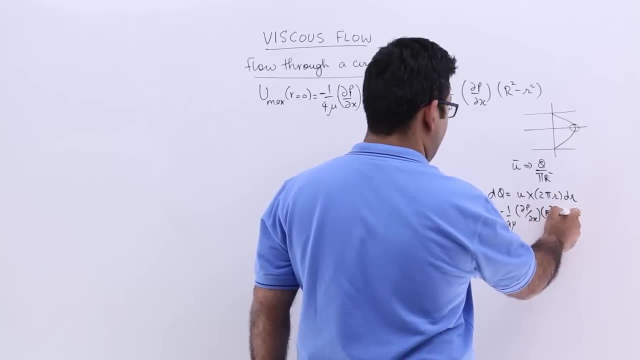 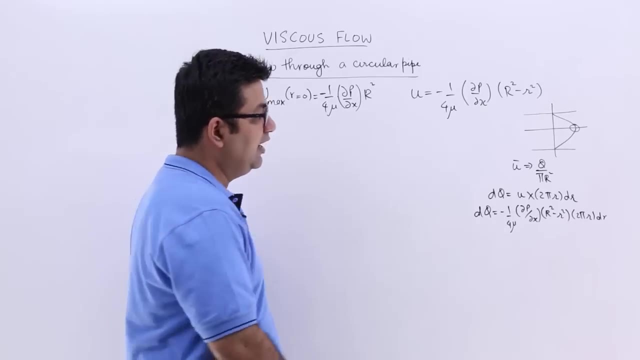 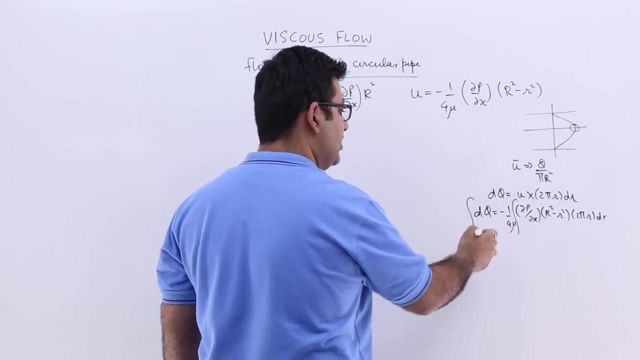 upon curly x into capital R square minus small r square into 2 pi r dr. So for the entire pipe you will have to integrate it for obvious reasons. So this would become integral, integral on both sides. This will become q. So when you integrate it, 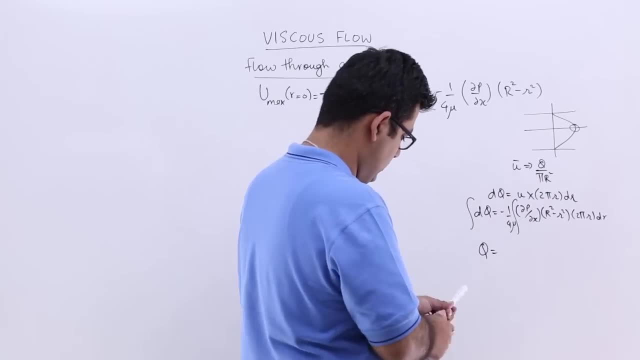 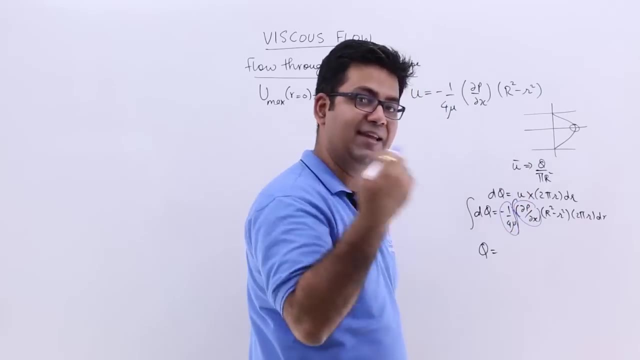 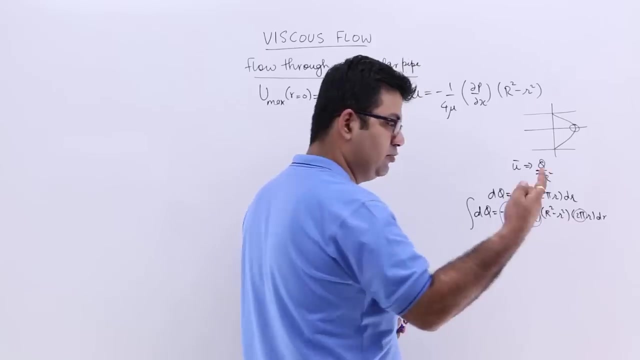 Okay. So when you integrate this you can take, you can take 1 upon 4 mu, this part. You can take curly p by curly x out and you can take 2 pi also as a common value. You will get R minus- sorry, capital, R square minus small r square into r dr. 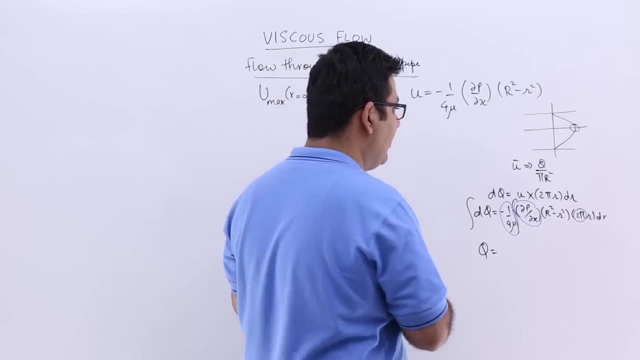 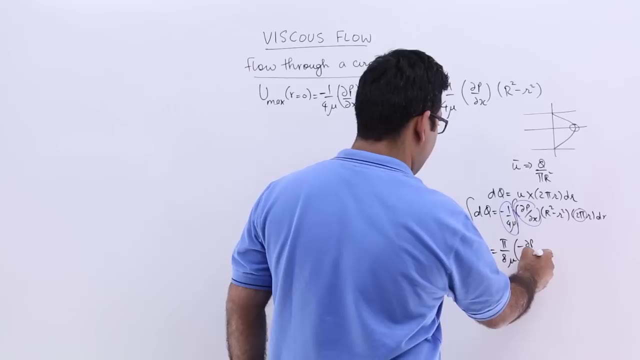 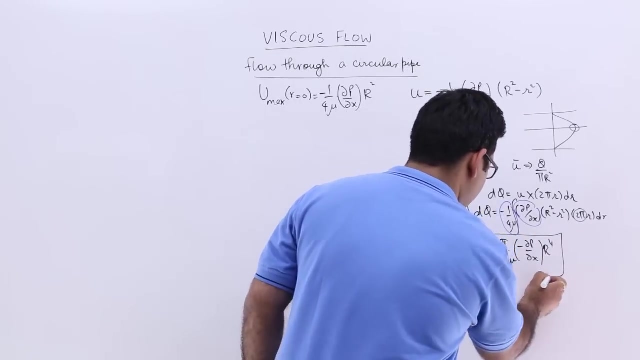 So when you integrate that part, the entire value will become pi upon 8 mu into minus r square. Okay, So this would become 8 into minus curly p upon curly x into capital R to the power 4.. So this is the final relation that you will get after integrating that equation. 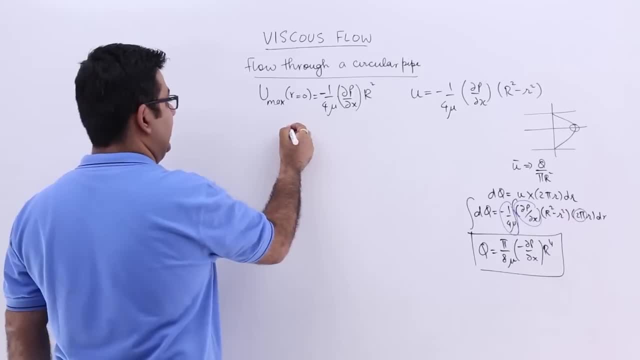 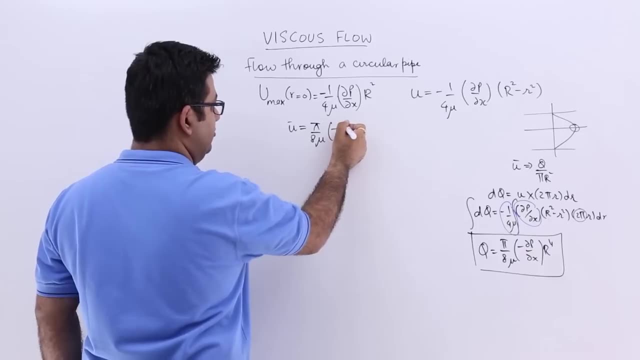 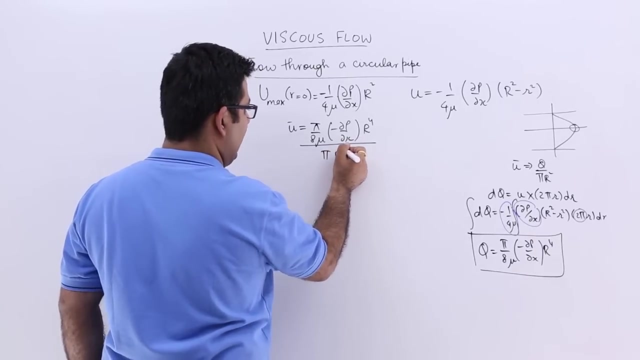 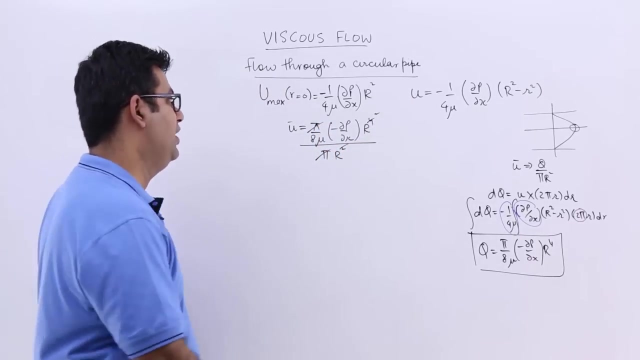 So to find out the average velocity that is u bar, I will just divide those two terms. So pi upon 8 mu into minus curly p upon curly x into capital R, to the power 4 upon pi into 8 mu, power 4 upon pi into capital R square. I can straight away take off pi and two powers of. 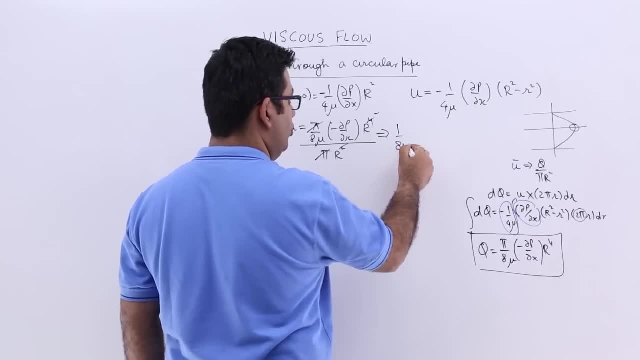 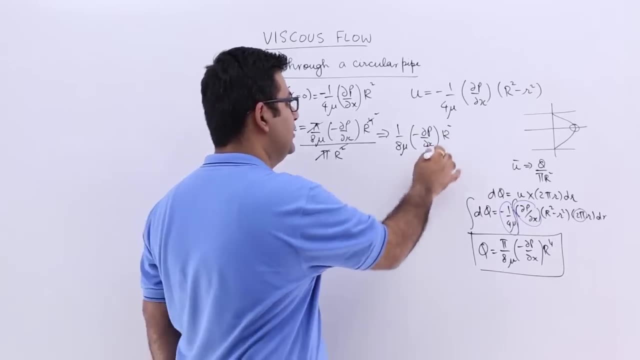 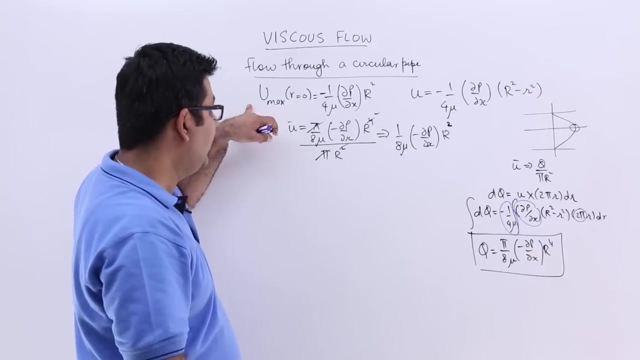 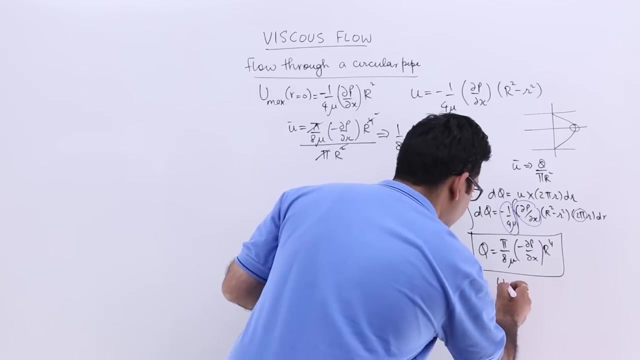 R. so you would get 1 upon 8 mu into curly p by curly x into R square. so that is the average velocity. if you take the ratio between the maximum velocity and the average velocity, it is clear that the ratio between these two would be two. so u max upon u dash is equal. 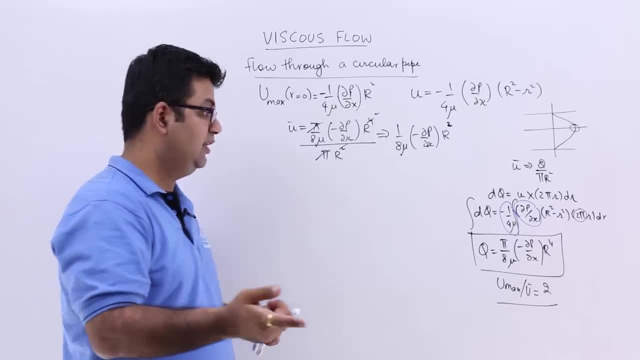 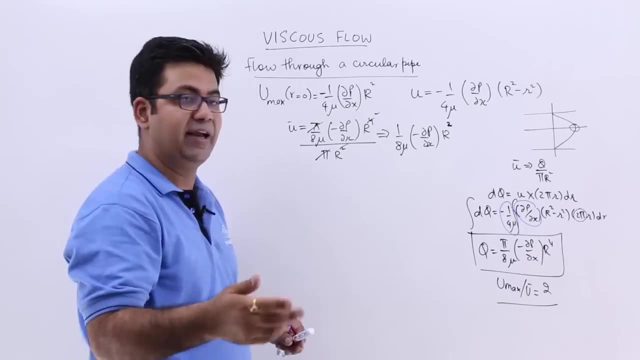 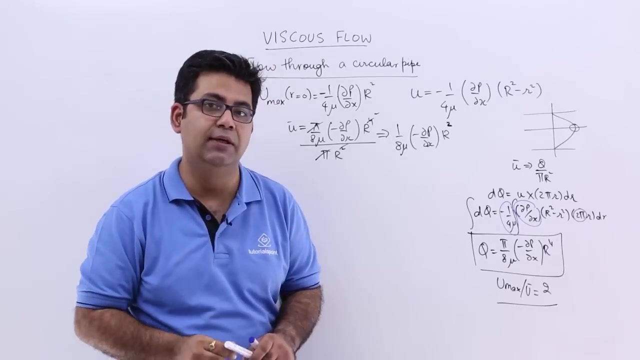 to 2, so maximum velocity is twice the average velocity in the case of viscous flow through a subtler pipe. okay, let's move forward and get some more. you know input from this, so we need to find out the pressure drop across a certain length, okay, so let me assume that. 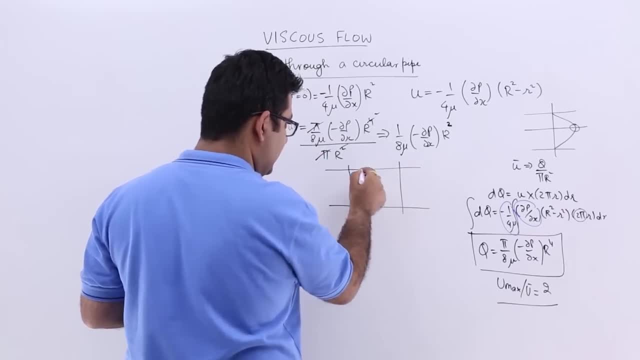 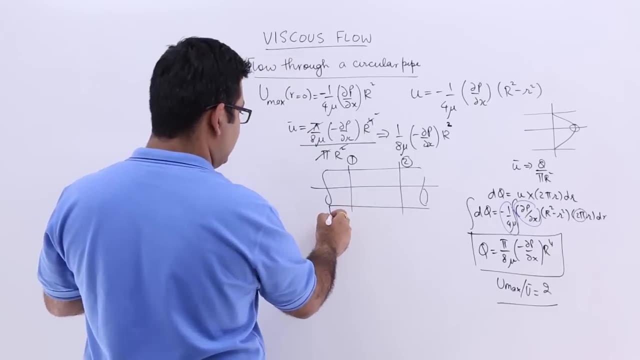 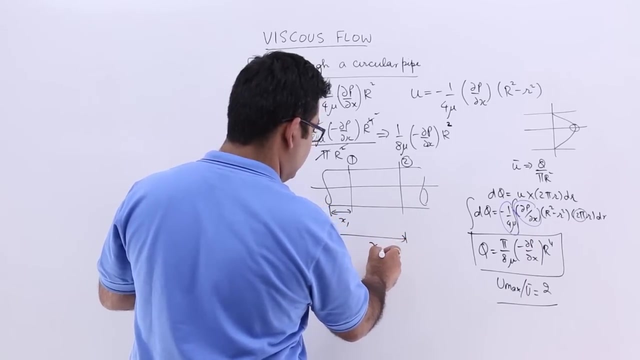 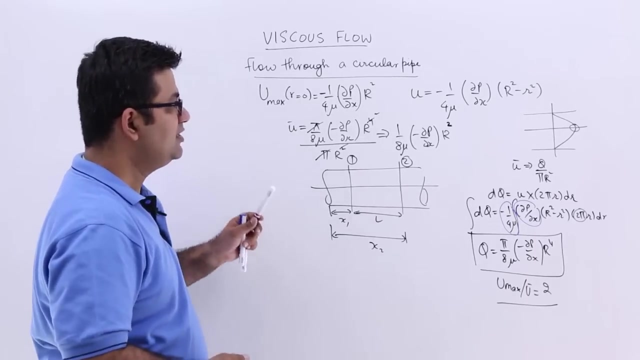 this is the pipe, two sections, section 1, section 2. okay, now let us say this is section at a distance x1 and this would be another section at distance x2. the distance between these two sections becomes capital L. okay, so if I start using, if I start using this particular 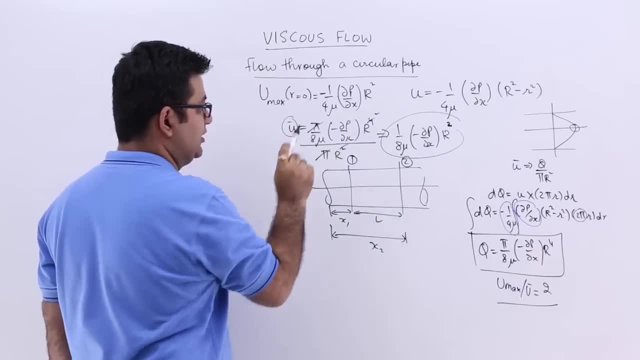 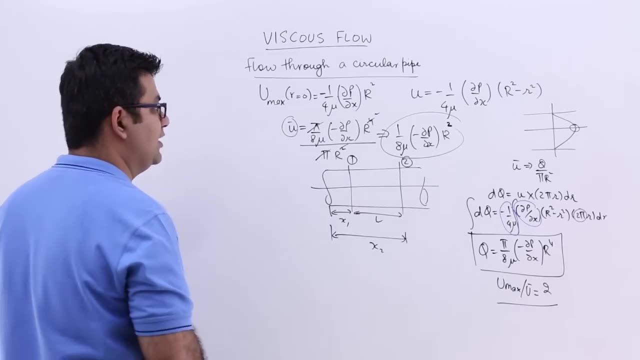 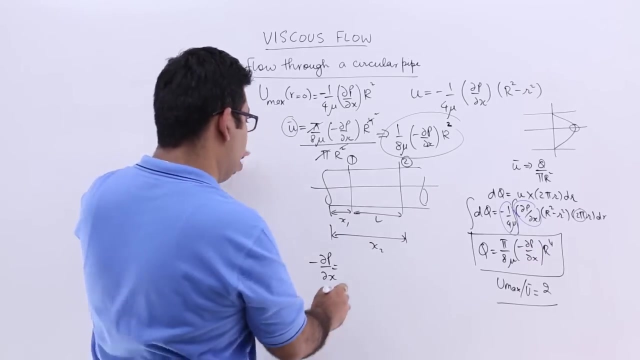 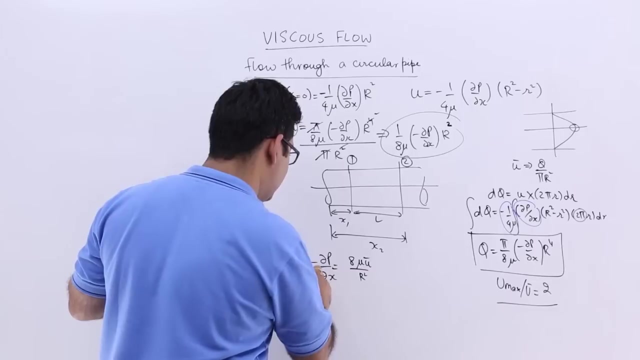 singular relationship, that is u dash, is equal to this. let's find out the value for curly p by curly x. so the value of curly p by curly x, or rather minus curly p upon curly x, this would be 8 mu into u bar upon capital r square. so this is what you get. let's integrate it. 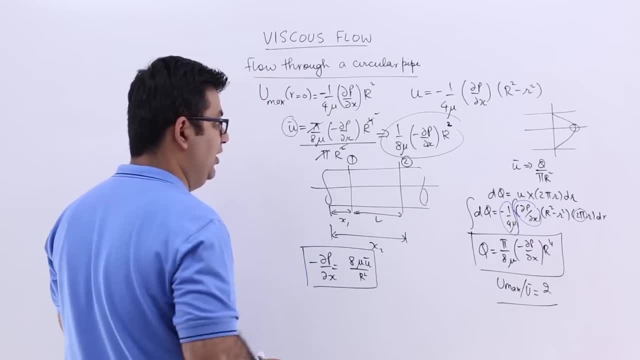 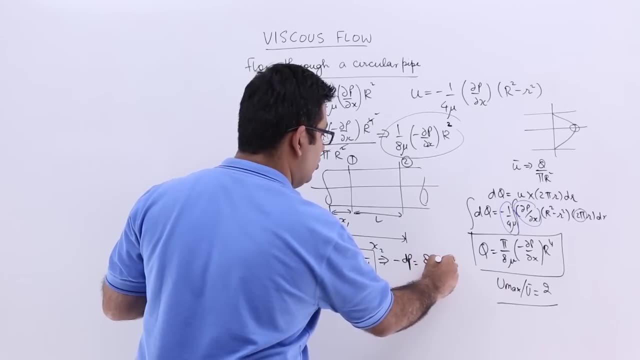 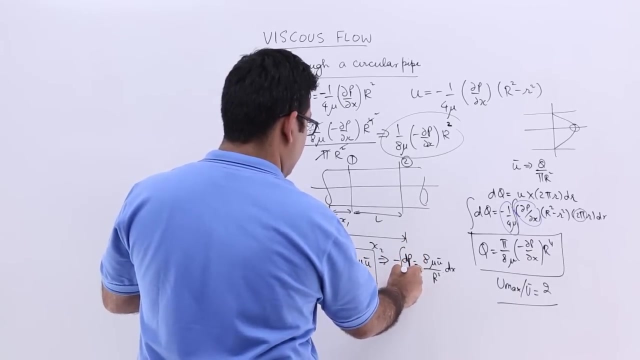 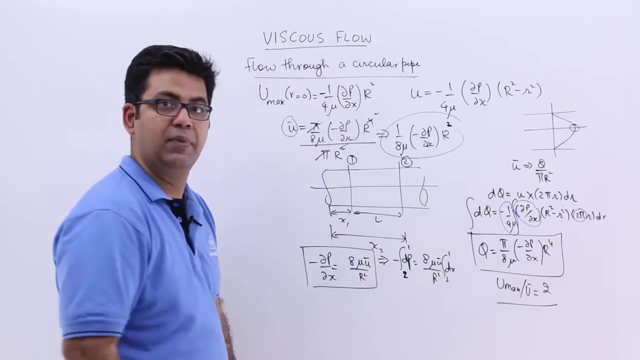 between sections 1 and 2. so this would be minus Dp is equal to 8 mu u. bar upon this into dx and i will have to integrate it between this and this also gets integrated between 2 and 1.. So i would get values P1 minus 2 and 1.. 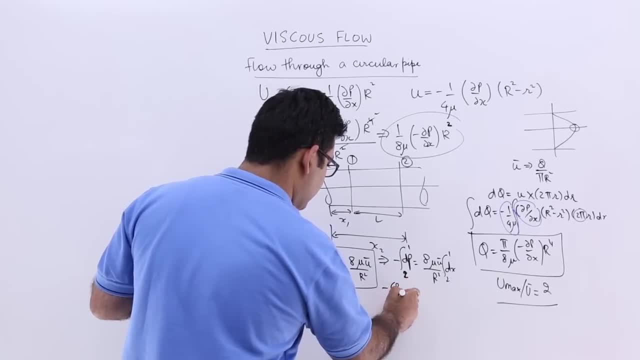 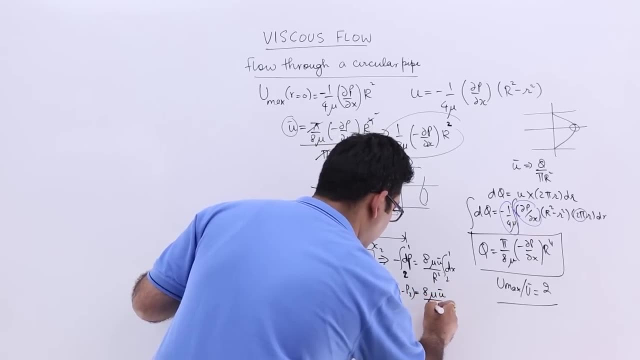 So what is u dot u, dot t us. So how it will happen? So in my particular table we used to have that dp and plus when is equal to 6 plus X, dp minus p2 or minus p1 minus p2. in brackets, this would be 8 mu u bar upon r square into. 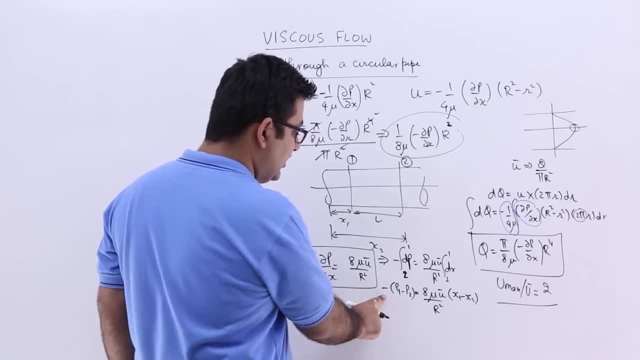 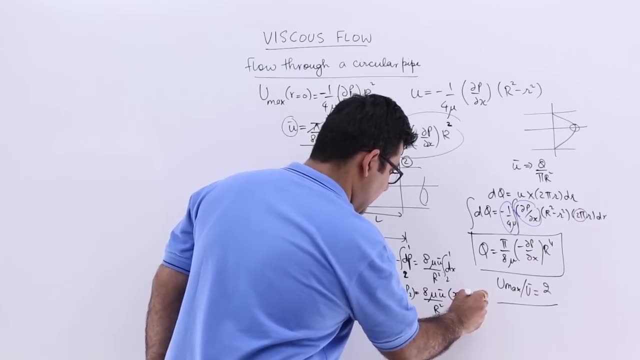 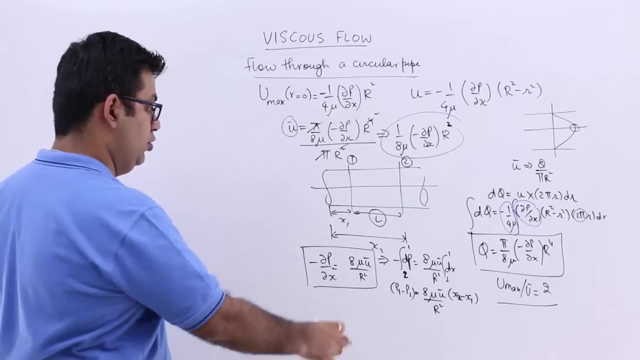 x1 minus x2. so let me take this negative sign on to that side and that is going to give you x2 minus x1.. Now what is x2 minus x1?? x2 minus x1, that is l, so you will get p1 minus. 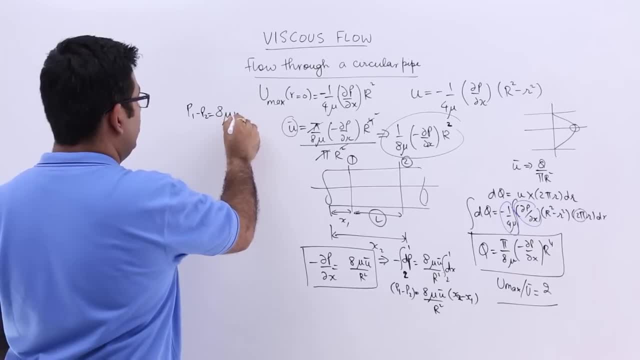 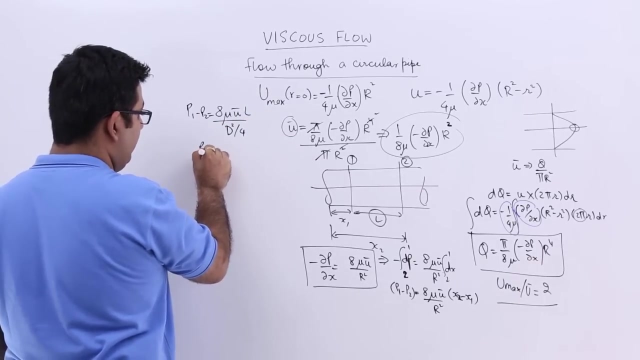 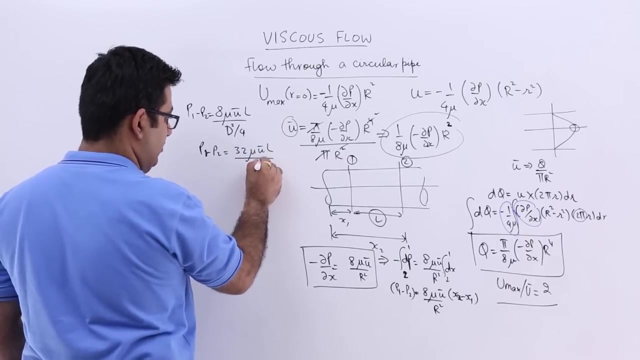 p2 is equal to 8 mu? u bar into l upon capital r square, which is d by 2 whole square, which will give you d square upon four. you take this on top so you get p2 minus p2 into r r square. or p1 minus p2 is equal to 32 times mu into u bar l upon d square. Now if I want to find 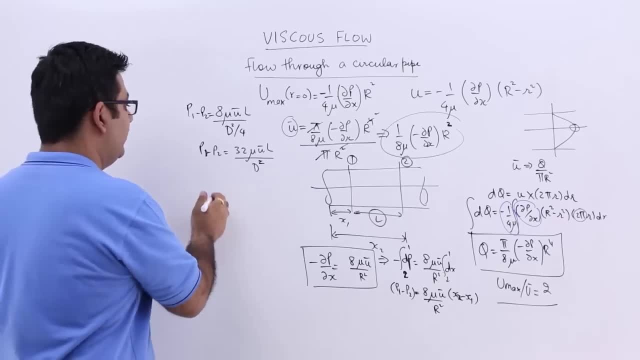 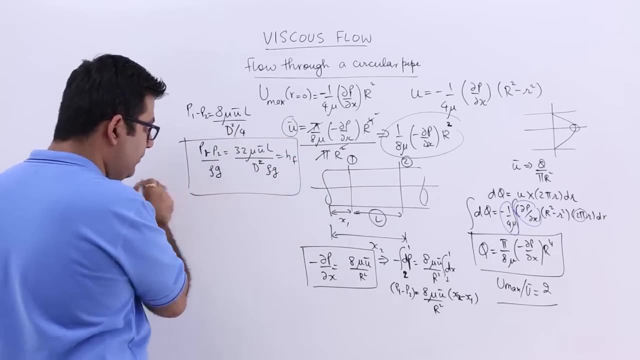 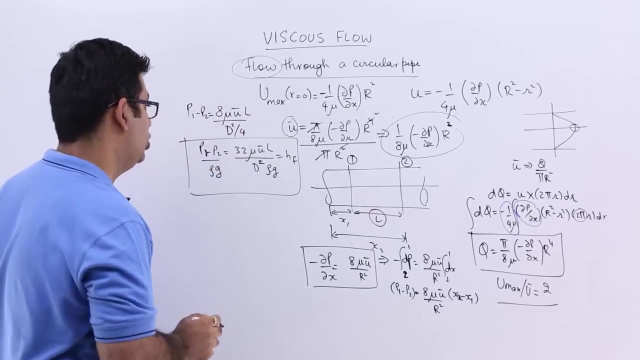 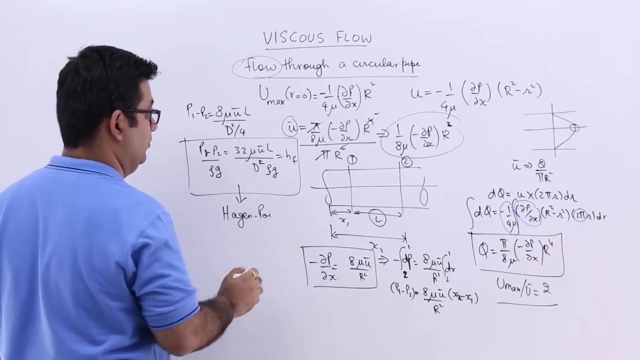 out the pressure head drop, I will have to divide both sides by rho g. This is hf, So this is the pressure head drop in this pipe in which you have a viscous flow happening. ok, So this equation has a name, which is called the Hagen Poiseuille's theorem or Hagen Poiseuille. 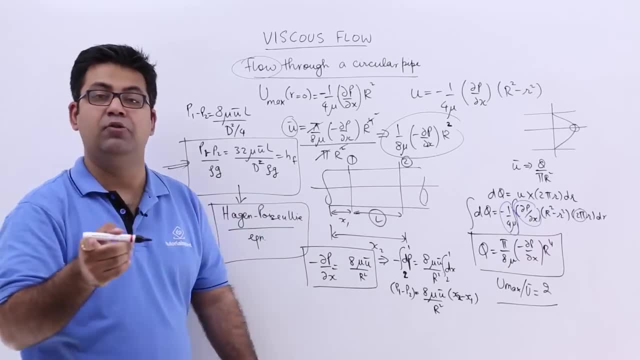 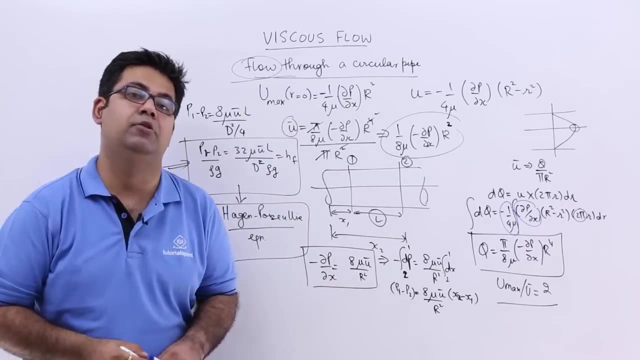 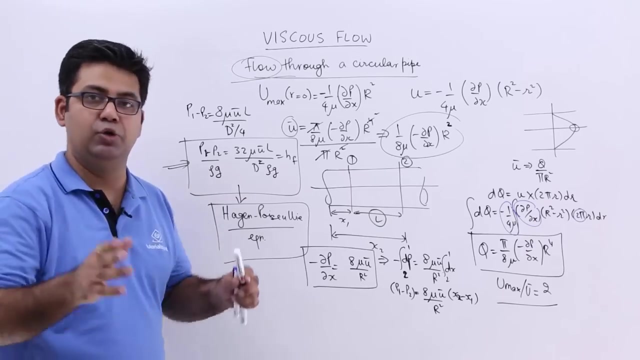 equation- So make a note of this- which is used to find out the pressure drop across a certain length for a pipe which has a viscous flow happening through it. So this is a pretty long analysis that we have done. This is the final result that you should remember. This is also one of the results that is worth. 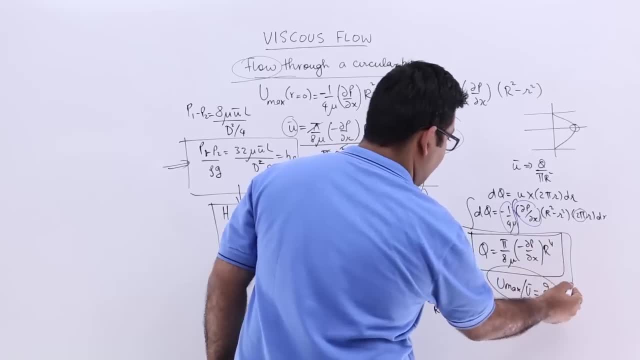 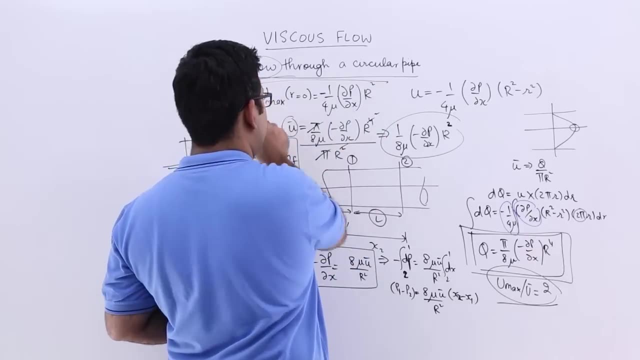 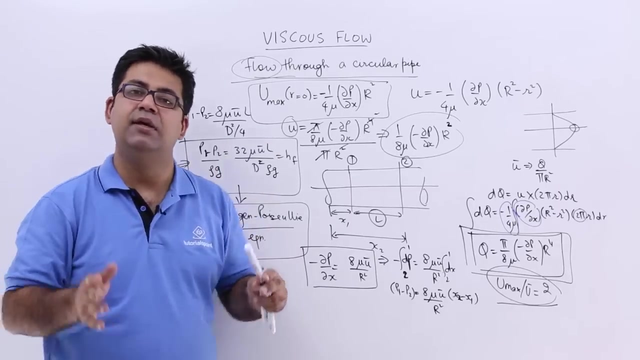 remembering. You should also remember the value of the flow rate happening through this pipe, ok, and the maximum velocity and the, but obviously the shear stress variation also. So I hope you understood this entire analysis. Now let's move on to the next video and talk. 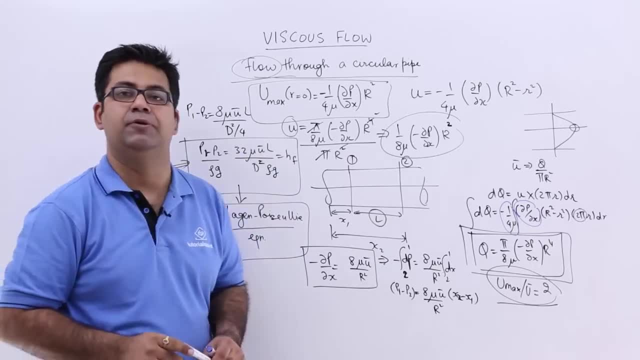 about some numerical applications of this concept. Thank you.